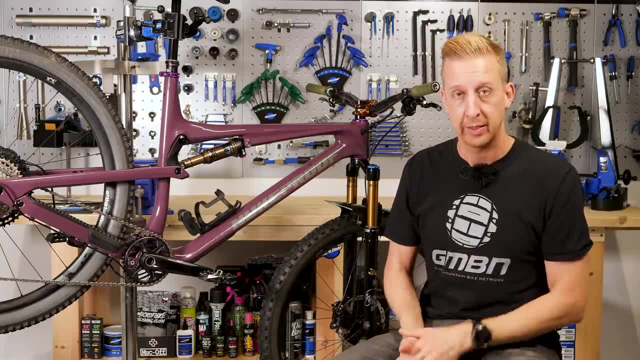 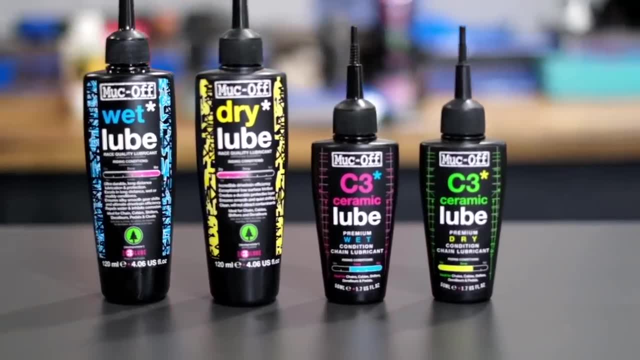 I'll give it a full once over and then I'll store it away. Now, before I go for my next ride, the one thing I will do is lubricate the chain. This is something you do want to do every single ride. Now I try and do this 10 minutes before I go and just leave the lube to work its way in. 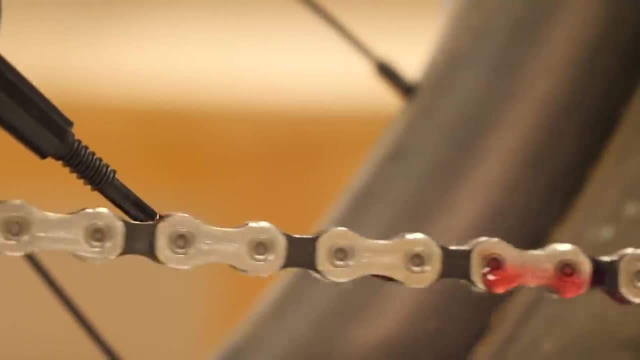 and then I wipe off any excess. If you just lube the chain and wipe it off, you're basically just getting rid of the lube you've just put on. Give it a bit of time to work its way in, Don't forget. 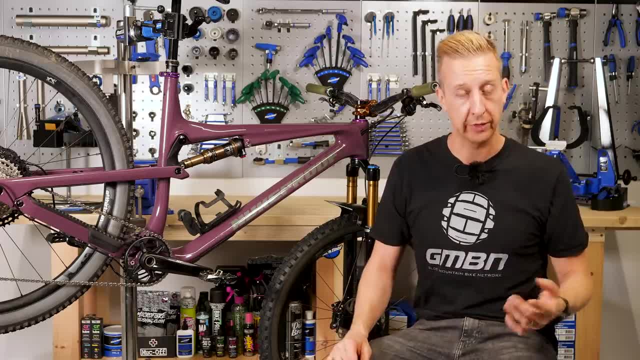 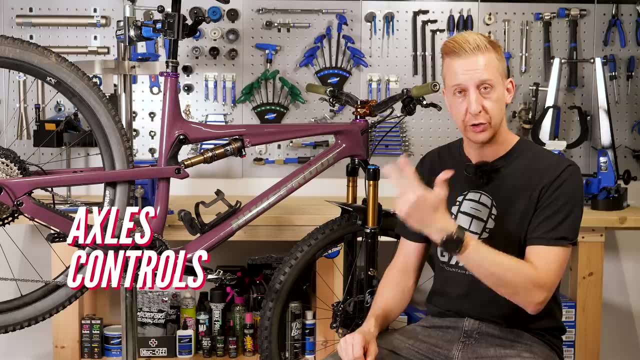 after every ride. it's pretty much just a sense check because you're going to know when you ride the sorts of things that might not be quite right, that you might need to pay attention to for your next one: Axles, controls, chain- they're the main things between every ride. 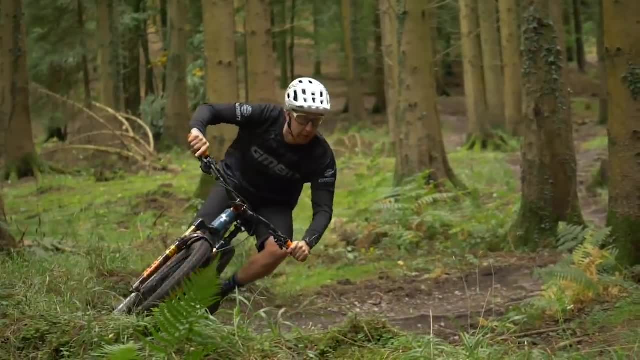 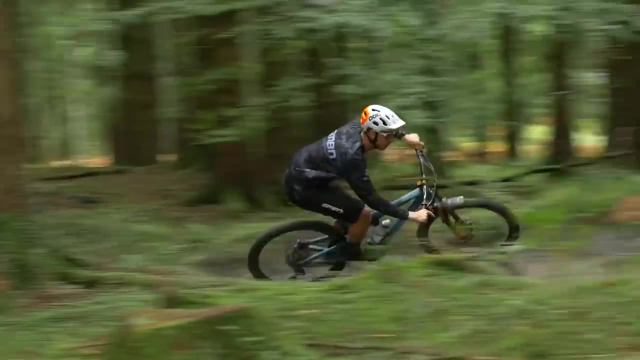 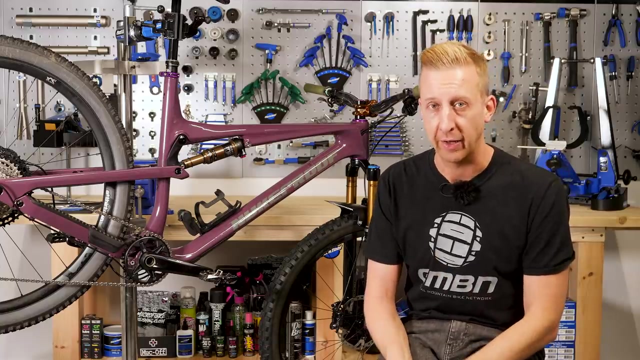 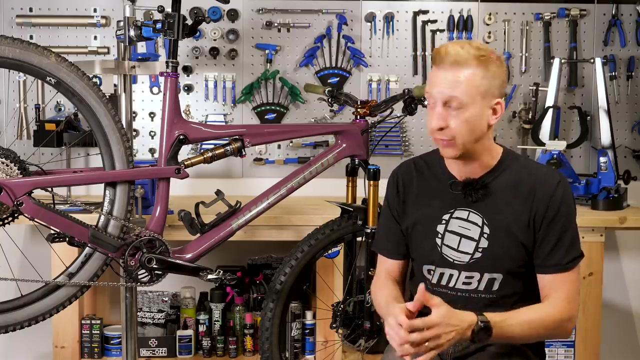 Now, this is based on someone that rides more than once a week, so perhaps two or three times a week. Now, of course, you're going to need to do this. on top of just lubing your chain and the basic stuff you'd do after a single ride, There's a number of things that you're going to need to. 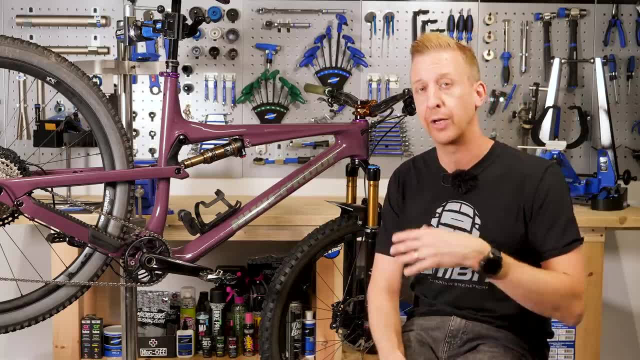 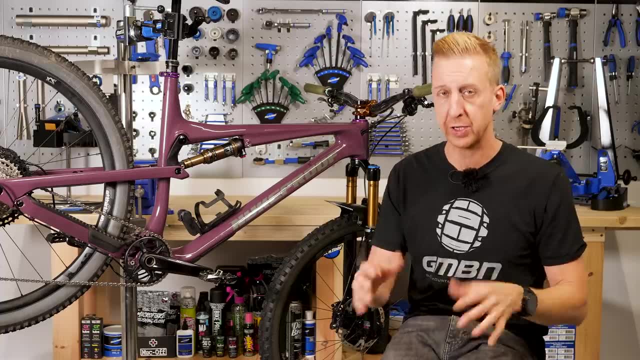 do to make sure your bike is safe. You think that riding a mountain bike in off-road terrain it's quite demanding on the bike, so it's unsurprising that you're going to get some issues here and there. Now, first up, start off with the controls. Check your brake levers for 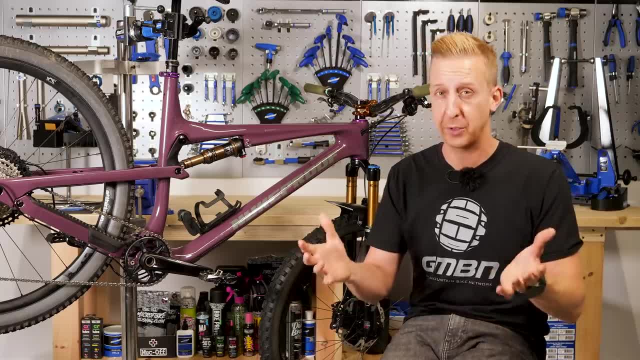 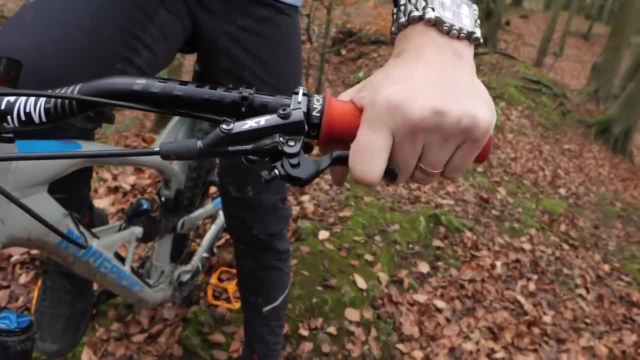 consistency. Give them a good feel. After all, your brakes are probably the most important part of the bike because it's a safety item. See how they feel. monitor them in between rides to make sure they're not pulling too far to the bar- stuff like that. Check your brake pads as well. 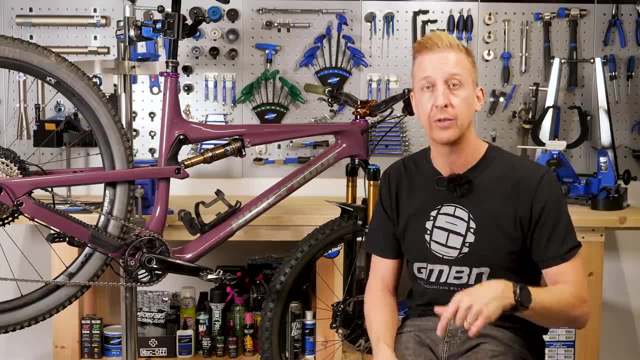 Now, this will depend on how heavy you are, how heavy on the brakes you are, The style of brakes, the style of brake pads. you're going to want to make sure that you're not pulling too hard. You have the mud and the weather conditions that you're riding and they're all going to. 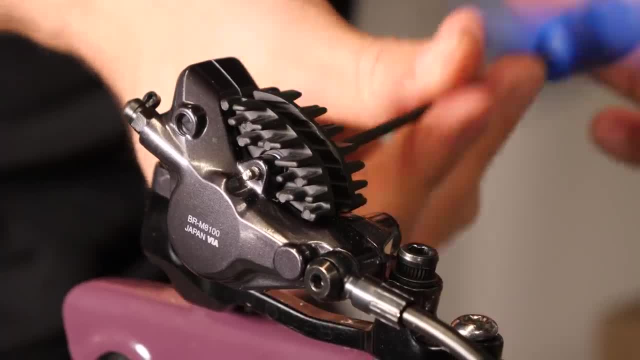 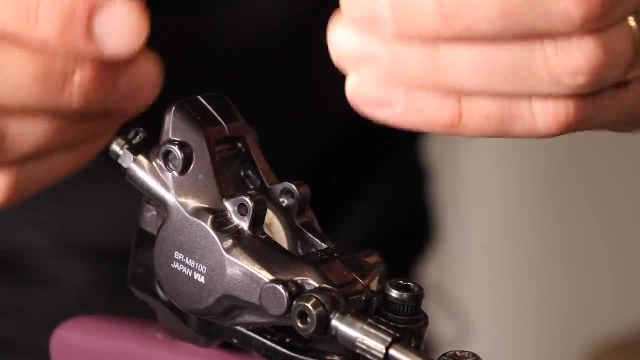 wear at slightly different rates and you can't guess this. You have to inspect them physically. Take your wheels out. have a look at the brake pads. You can just glance in there, but it's also quite a sensible thing just to remove your brake pads. It literally takes two minutes to do. 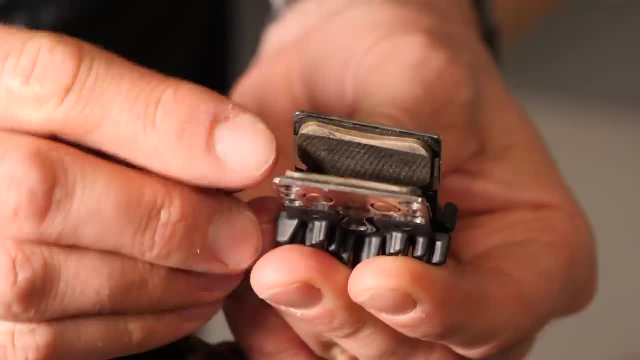 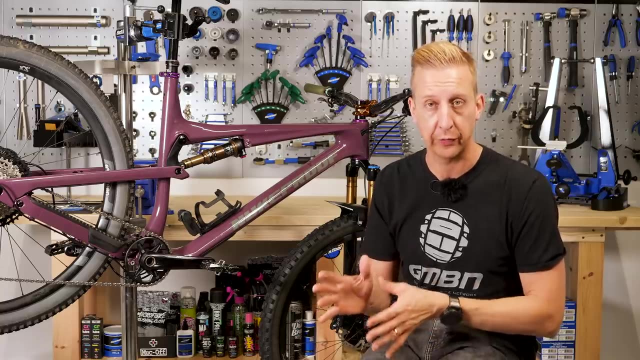 and you'll know where they are on the level of wear. You don't want to be braking on the backing plate. You want to make sure there's lots of pad material left on there When you put your wheels back into the bike after reinstalling your brake pads. just make sure. 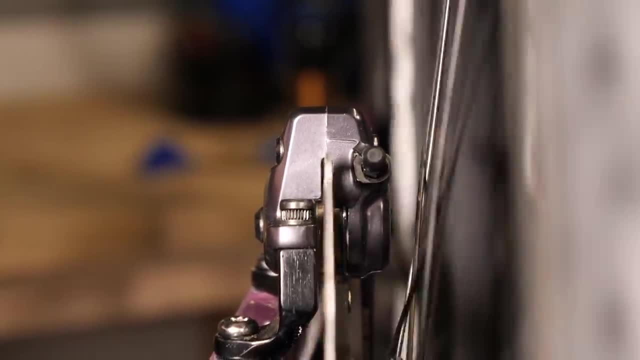 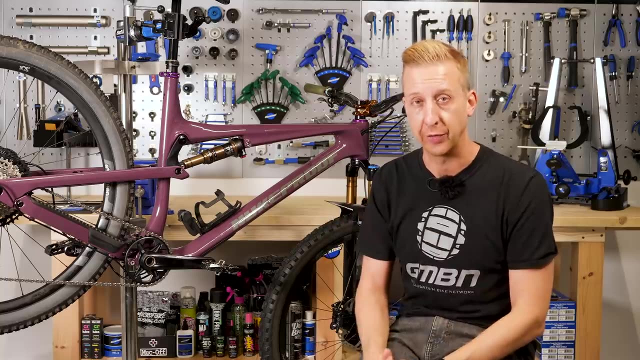 that your brake rotors aren't rubbing on the pads at all. It's common, actually, for your brake caliper to come out of alignment. They don't always stay completely true or your brake rotors can actually start bending a bit. Just make sure that they're running true and there's no hindrance. 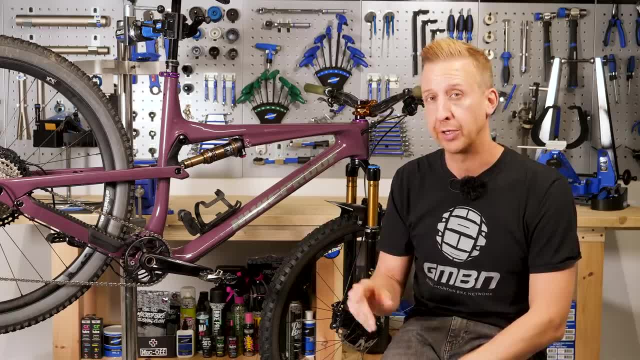 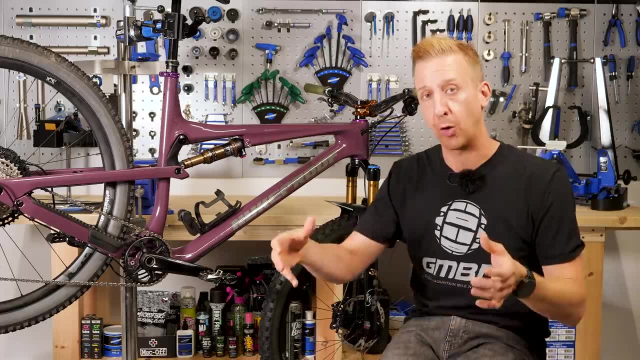 to the action Next up. a complete bolt check of the bike is a really good idea, but to start this, a good thing to do is to make sure your shock is unlocked, and the same with your fork. if you use the lockouts on them, Just drop your bike. Listen for any peculiar rattling. that sounds a bit. 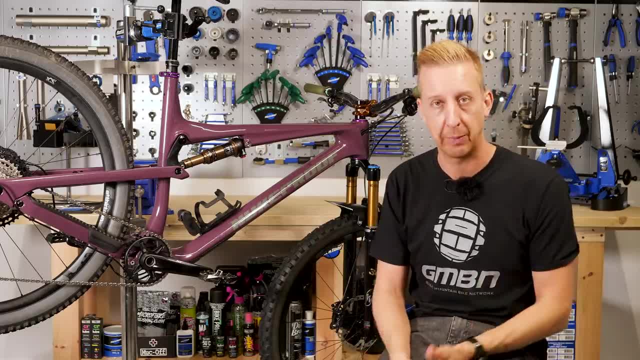 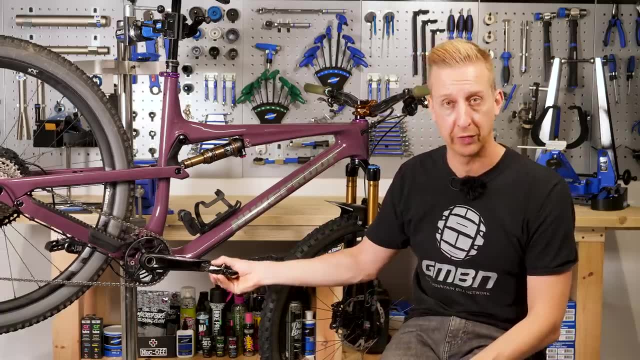 odd. Of course, your chain will be slapping and other things that make noise will typically do that, but this is where you're going to start hearing if things are a bit wrong. A classic one that you might hear is if your pedal rattles, suggesting your pedal is actually loose and might. 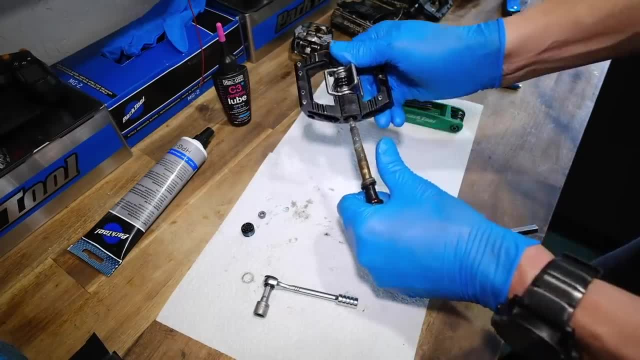 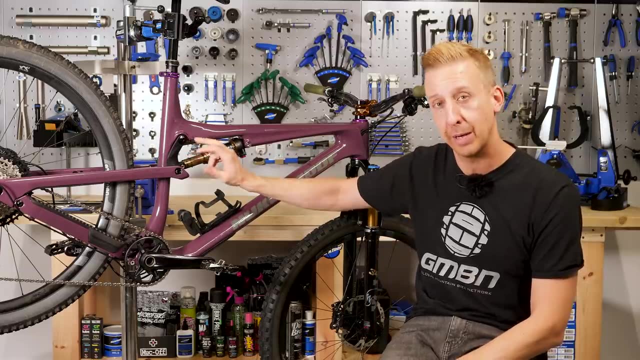 need some adjustment. Use your common sense, listen for the noises. if there are rattles, and chase them around the bike with an allen key and make sure you tighten things up. If it's anything like pivot hardware, make sure you tighten them to the torque settings as 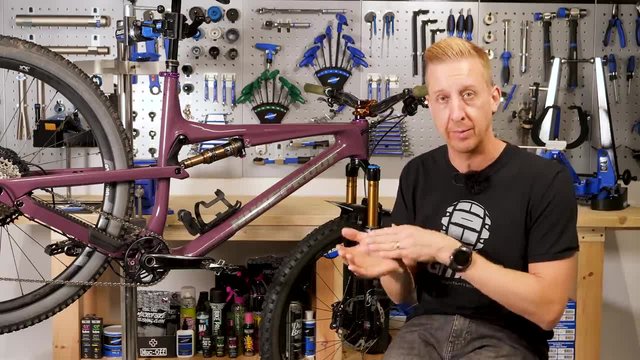 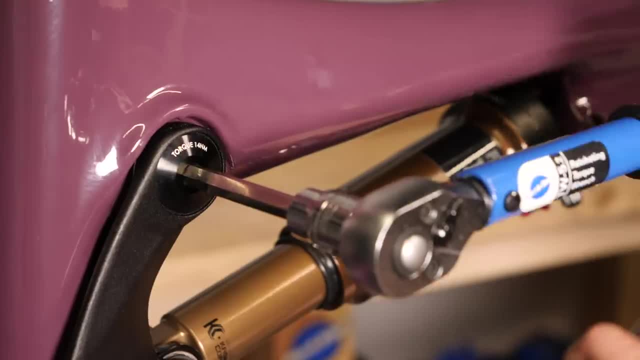 recommended, You think, the amount of strain that goes through the pivots of the frame when the suspension pivots are actually operating, and then the forces of you riding that bike. it's unsurprising from time to time that they will work loose, even with thread lock on them. 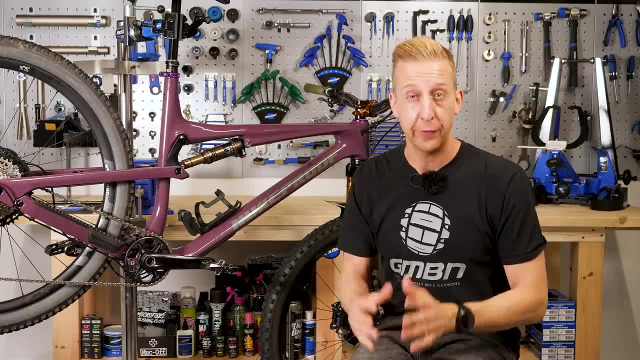 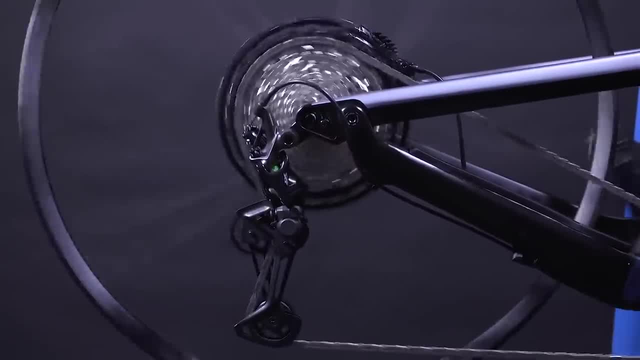 so just take a bit of care and give them a check. If you're able to get your bike in the work stand, give the gears a once over. just make sure they're good. To be honest, gears these days are pretty good. Once you've indexed them, you don't really have to adjust. 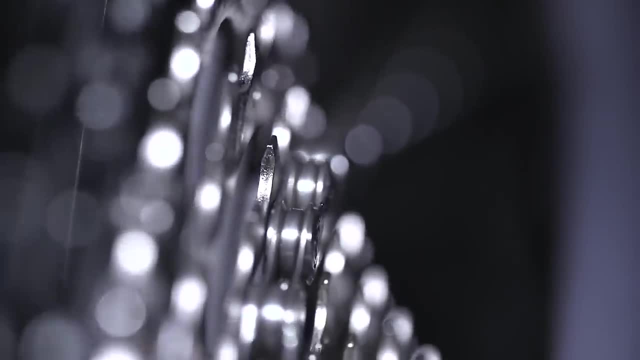 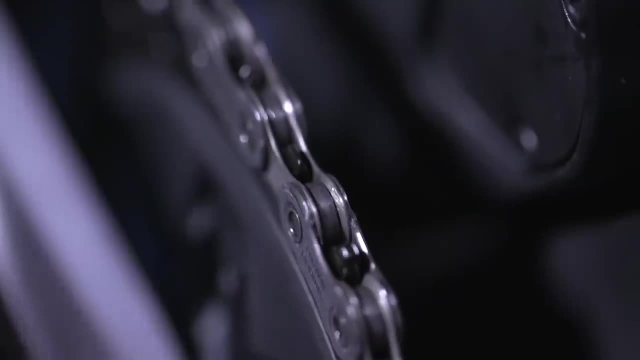 much more than just a little turn of the barrel, adjust if your gears aren't quite playing ball, but it's always worth a visual inspection. While you're at it, just check the chain as well. It does no harm to check every chain link. Follow from your join-in link all the way back. 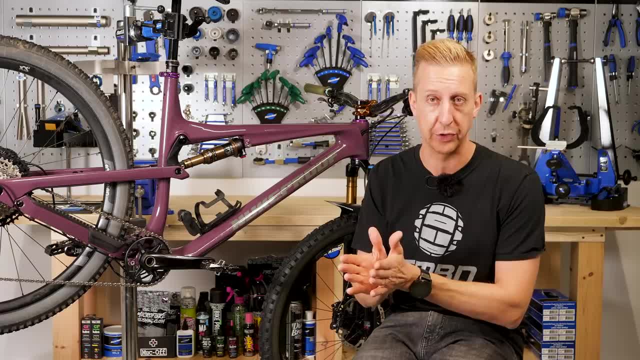 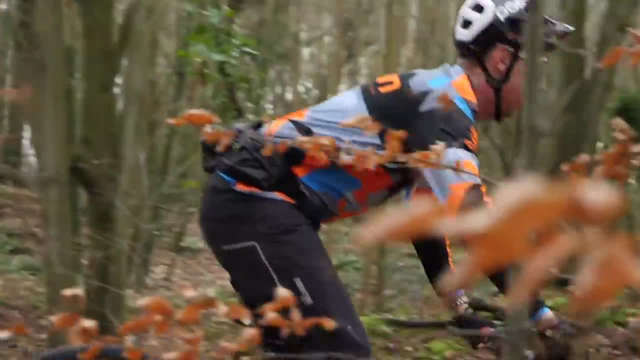 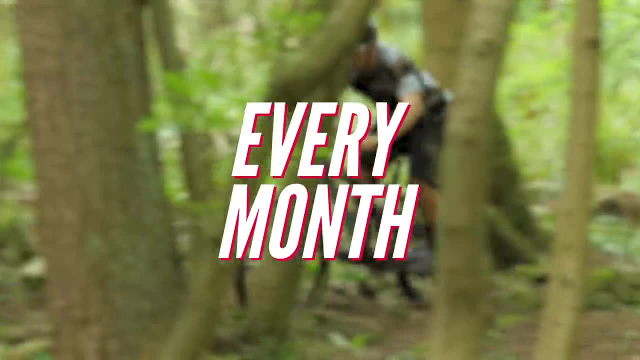 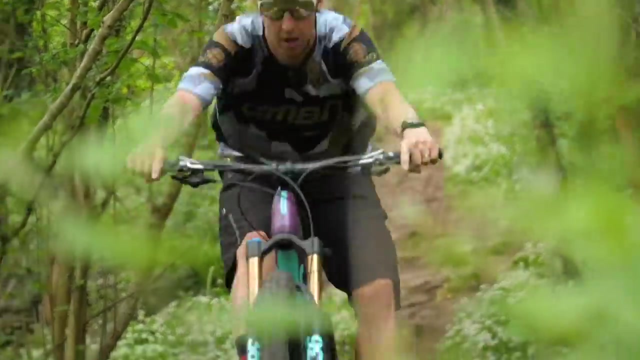 around again just to make sure there isn't anything that looked like it could turn into a broken chain. Trust me on this one: it really hurts when that does happen. Okay, now we're onto monthly, and this really is where things start changing from the daily and the weekly basis, because if you're a regular rider, 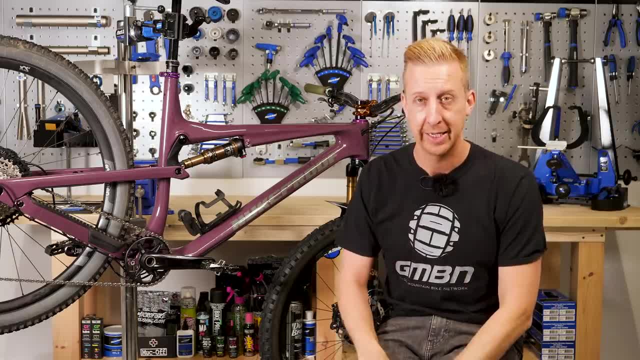 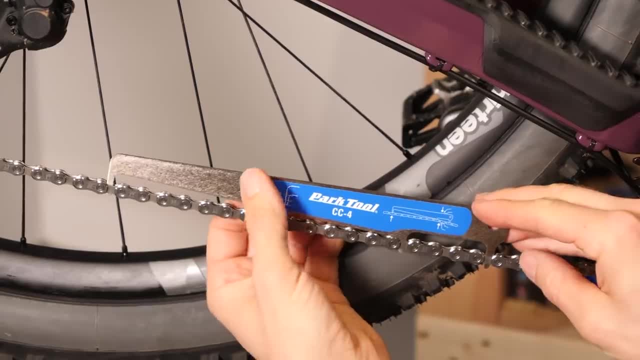 things will wear out and you need to make sure it's not going to cost you any money. The first thing you want to make sure you're doing on a monthly basis is checking your chain. This is designed to check the length of a chain. There's something known as chain stretch. 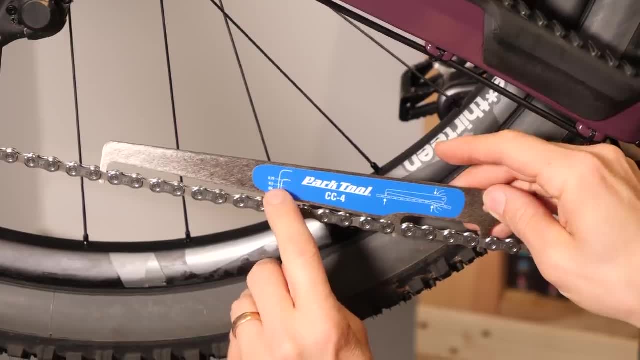 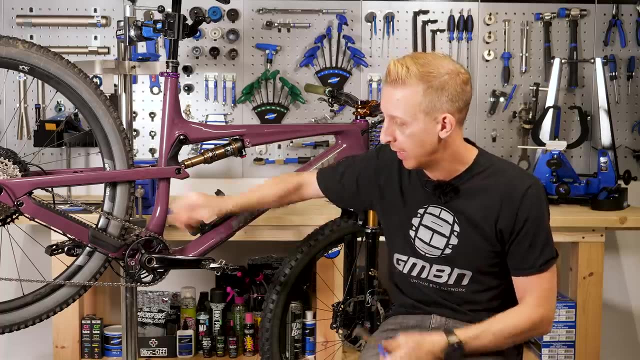 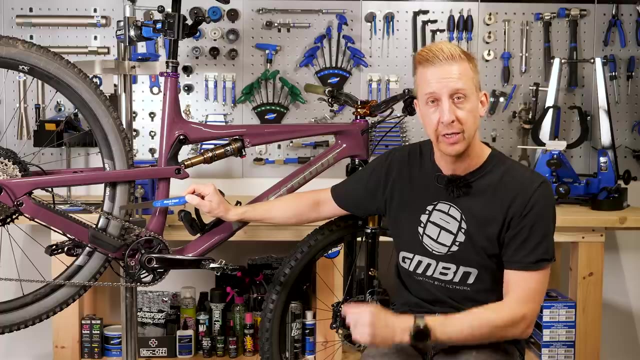 which is a bit of a misleading term. Chains are measured from the pin to pin. That's known as the pitch of the chain. The pitch can actually grow as the chain wears through time. What happens is the chain itself doesn't stretch, but the rollers that go around the pin on the inside they actually. 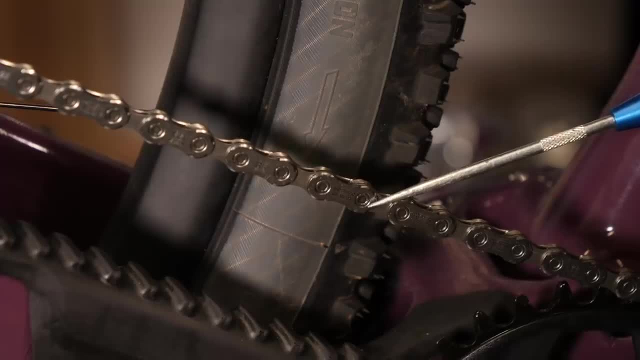 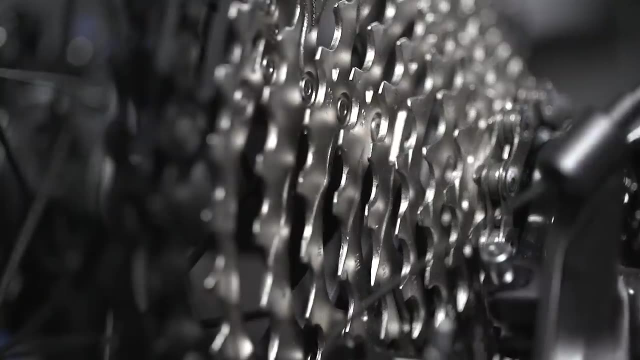 wear out from the middle. They kind of like bore out. As that happens, the pitch effectively changes slightly. The effect of that is that the rollers on the chain don't line up correctly in the troughs of the teeth, whether it's on the chain wheel at the front or in your cassette at the rear. 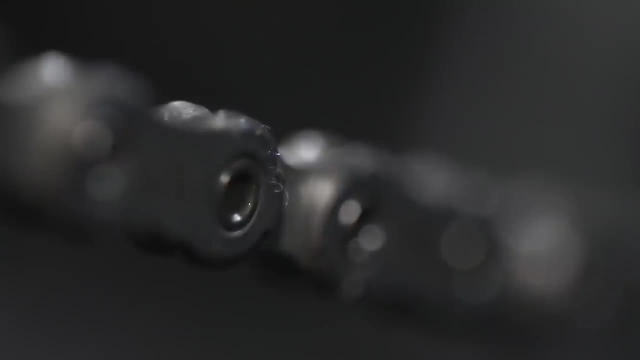 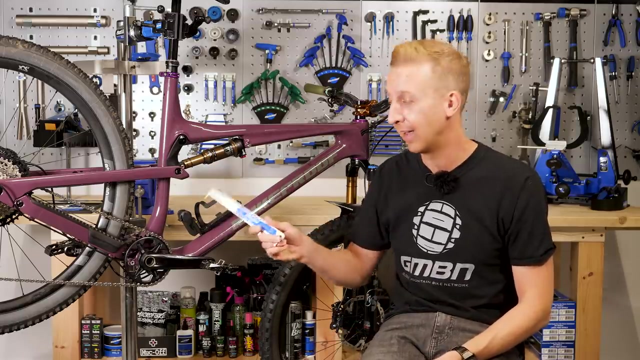 By doing that, it's just going to wear the wrong part of those teeth. When your chain wears, it's really important to get that replaced as soon as you can. The chain replacing it is a lot cheaper, Speaker 1, than having to replace a chain and a cassette and potentially chain at the same time. 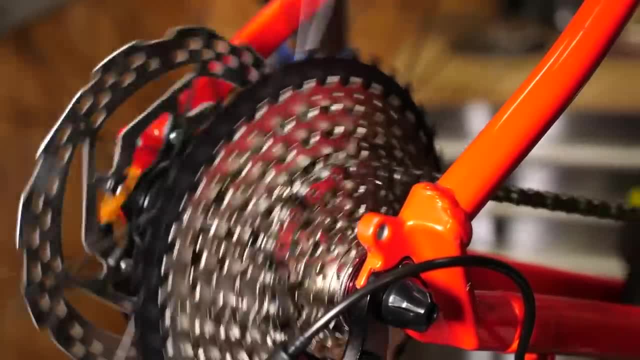 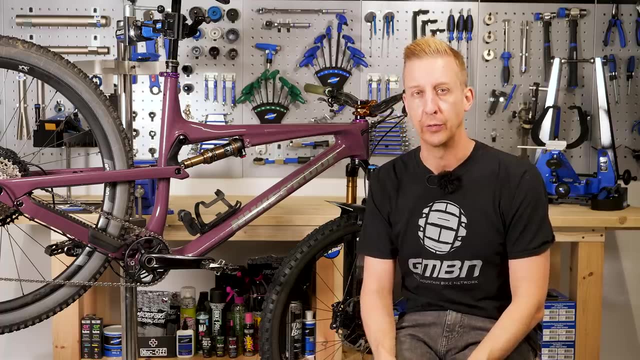 If you do this right, you can get two, sometimes even three chains to one cassette, all depending on how finicky you are with your maintenance. Have a good visual inspection of your wheels Now. work your way around, fill the spokes. 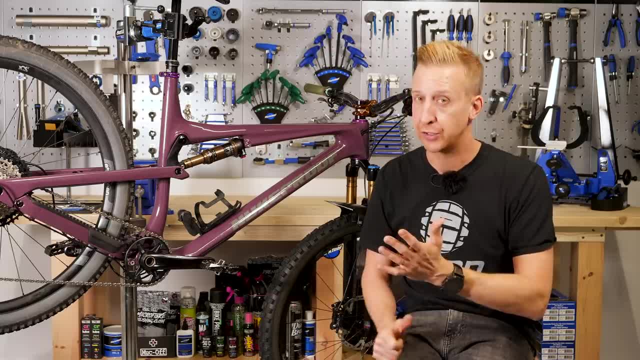 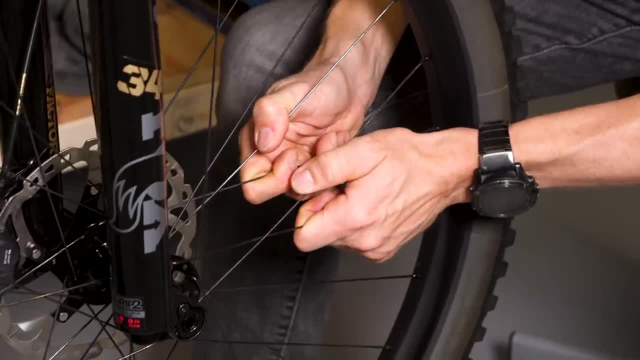 You're trying to feel for anything that's loose. If they're creaking or anything like that, the chances are, because of the fact that wheels, under load, they do bend around a bit, The spokes can rub together and cause a bit of a creaking noise. but that could be down to a loose spoke. 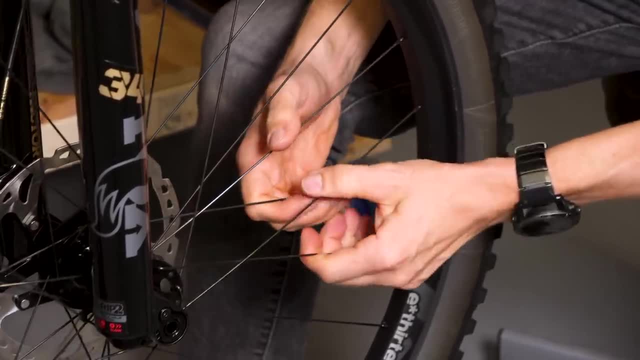 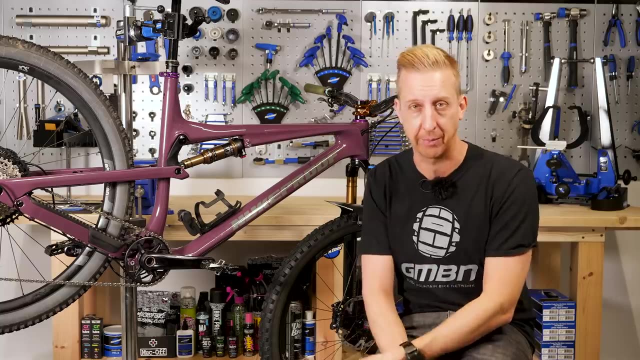 Use your common sense. if you're not used to building or truing wheels. If something feels abnormally loose, then you should just nip it up. Don't go too tight though. If you're unsure about this, there's definitely something for the bike shop. If it's abnormally loose, definitely nip. 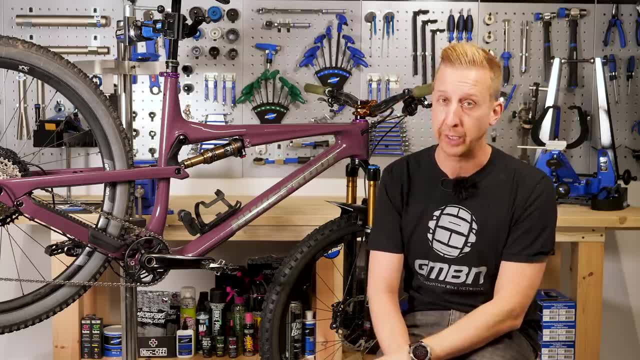 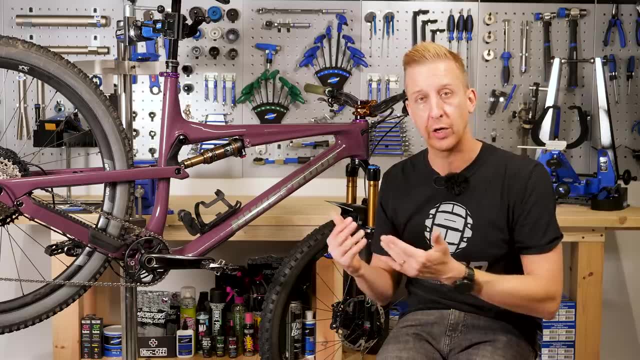 it up tight and perhaps make a marking just so you can reference which one it is. so when you take it to the bike shop you can show them and they'll be able to take care of that. Now work your way around your tires. Look at all the sidewalls. Make sure there's no bulges or it's not unseated, or if there's any slashes in the sidewalls, Make sure there's no bulges or it's not unseated. or if there's any slashes in the sidewalls, Make sure there's no bulges or it's not unseated. or if there's any slashes in. 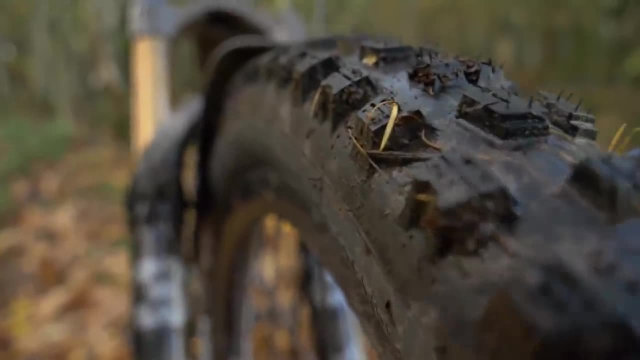 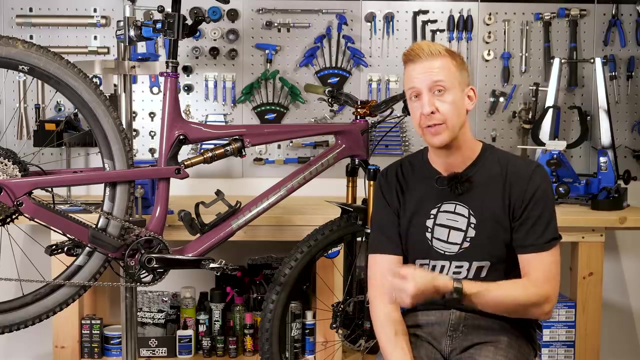 the casing, work your way around. Quite often it's common to find nails and screws and all sorts of big thorns and things that have worked their way into the tire. Now's the chance to take them out and, if need be, to fix that tire. Get it done now and it won't cause you hassle on a longer. 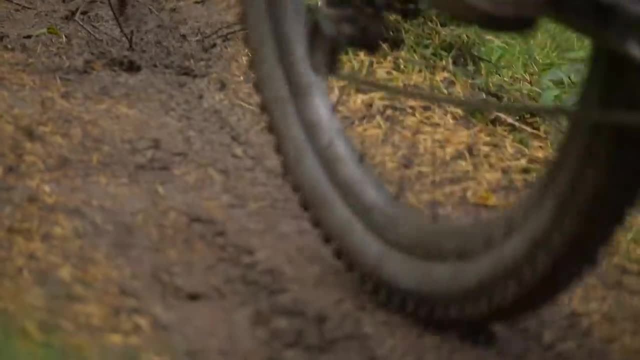 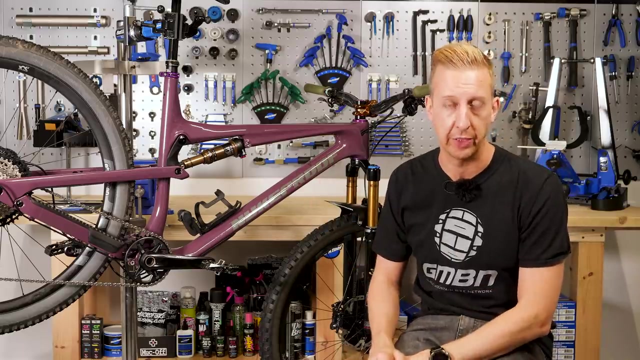 later ride. Finally, the last essential thing you really need to be doing a bit of minor servicing to be fair on a monthly basis- is to pay attention to your suspension units Now. the seat post actually counts as one of those because it's a telescopic. 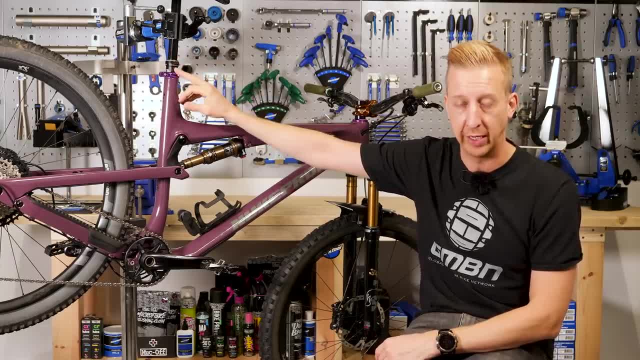 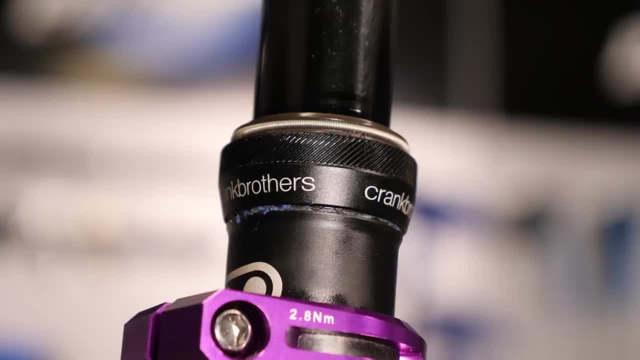 unit and in its nature it will ingest muck into here. At the very least you should be giving this a good, clean. apply some suspension lube on the outside of the seal and then basically drop your post a few times. motion it through the works and you'll notice that, if there's any, 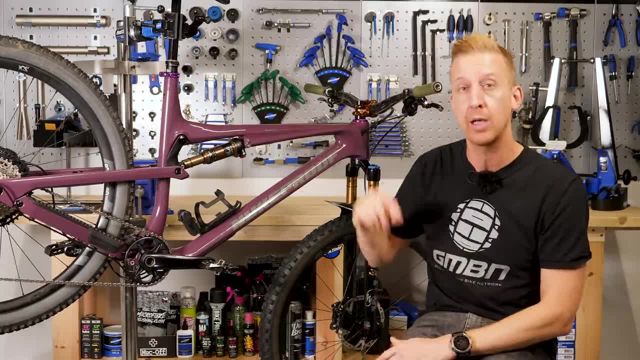 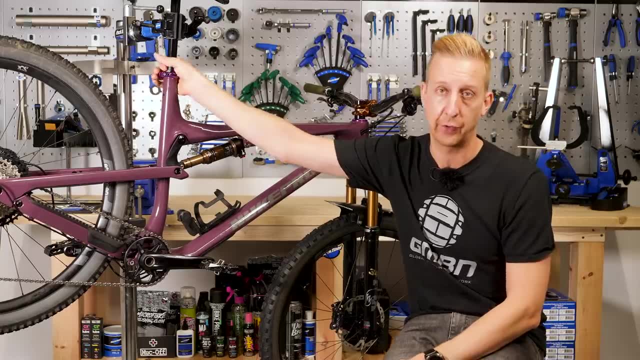 muck on the inside, the oil will actually pull it out. Wipe that away, put some fresh oil, do it again until it's nice and clean. If you're happy going a bit further, you can actually remove the top collar here just by loosening it. If I do that now, you'll be able to see You can directly. 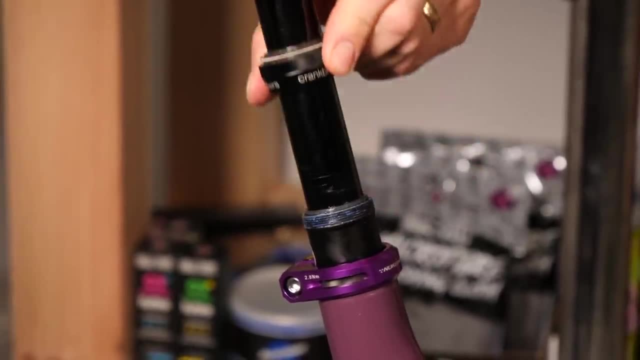 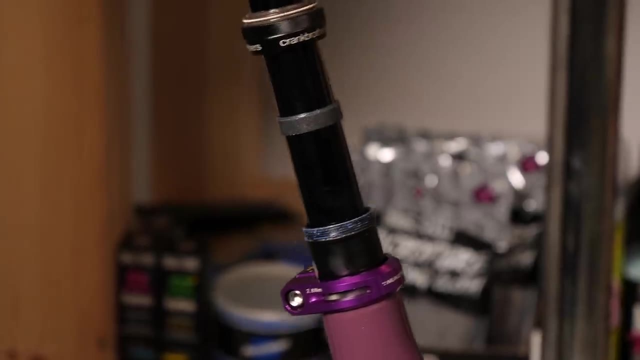 apply the oil underneath it, but it's always a good idea to cycle the post as you're doing this, and you'll find the bushing will just move up. Give it a good wipe. some suspension grease and a bit of suspension lubricant is a great idea for this. Same applies to your fork and shock. 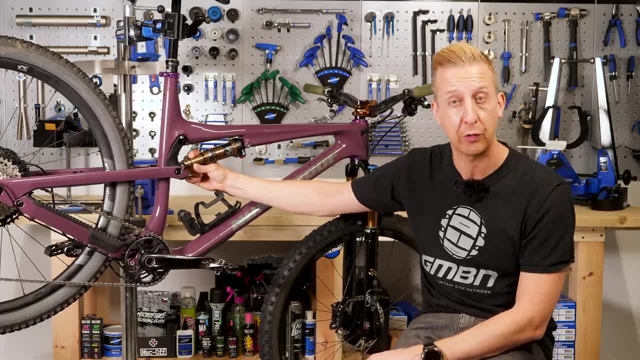 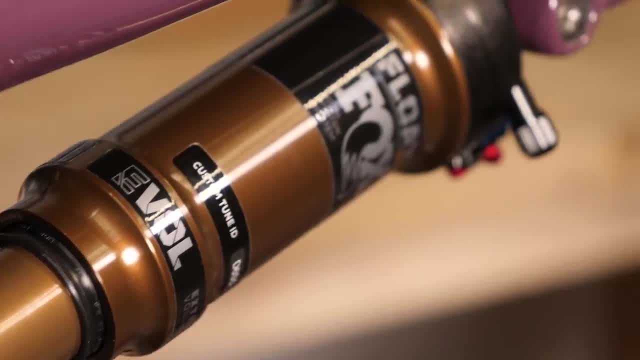 Look at the shock stanchion surface as well. Make sure there's no scratches or scuffs on it, Make sure it's nice and clean, and inspect the actual seal. Give it a good wipe down and make sure visually it's all in sound shape With the forks, though they're subject to a bit. 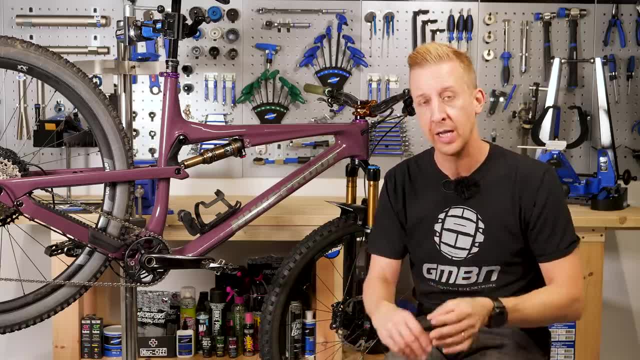 more abuse because they're not going to be able to get the oil out of the fork. They're going to get the oil out of the fork Because of the fact you've got all the stuff that flies off the front tire and the fork seals are basically facing upwards, which means muck can sit on them. 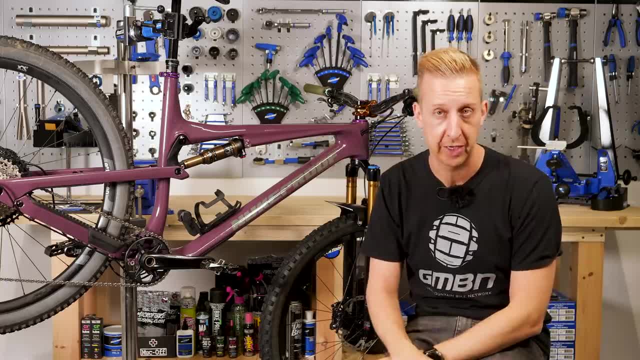 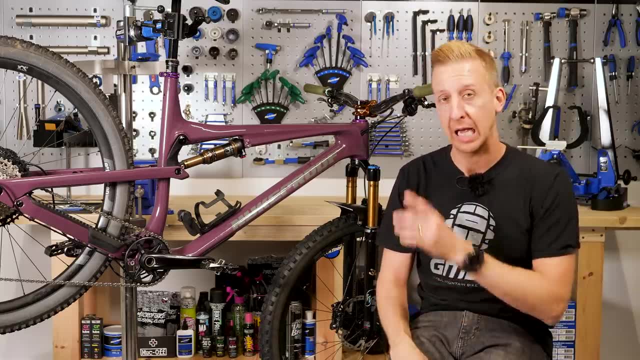 They naturally just ingest stuff into them, just like the dropper post does with the stuff that flicks off the rear tire. You want to make sure that your fork seals are as clean as possible and repeat the same process with them as you did with the dropper post: Put some suspension. 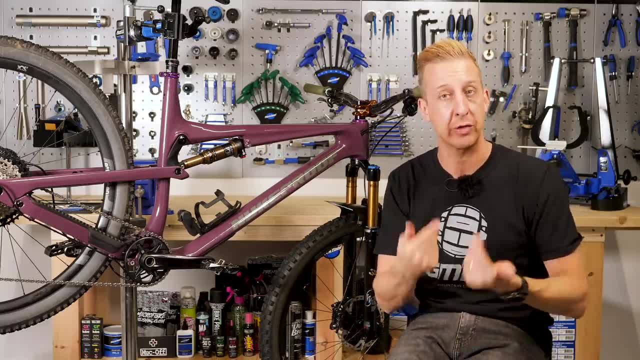 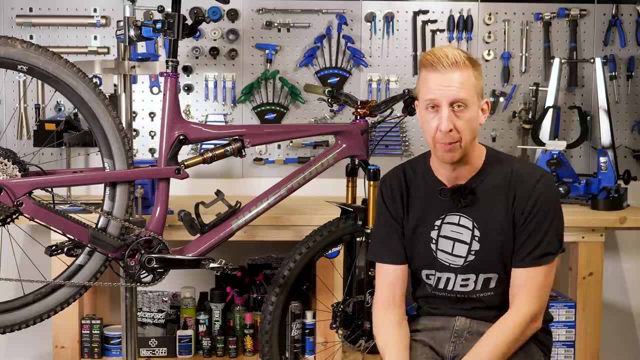 lubricant around the top of the seal. compress your forks a few times and it will naturally pull out some of the debris that's just under the seal. Clean them, repeat, clean, repeat and then do a fresh load just on the top. Make sure whatever suspension lubricant you're using, it can't get. 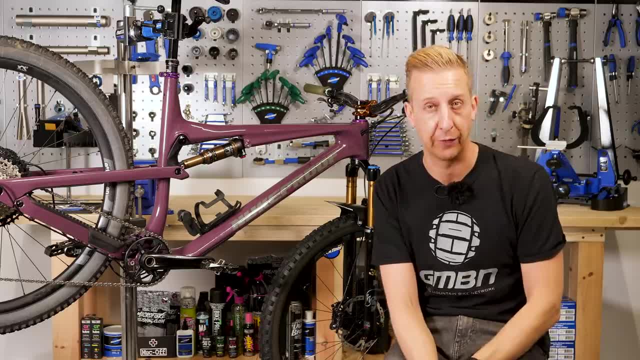 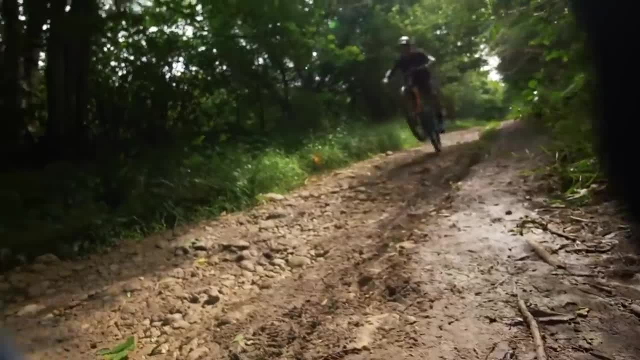 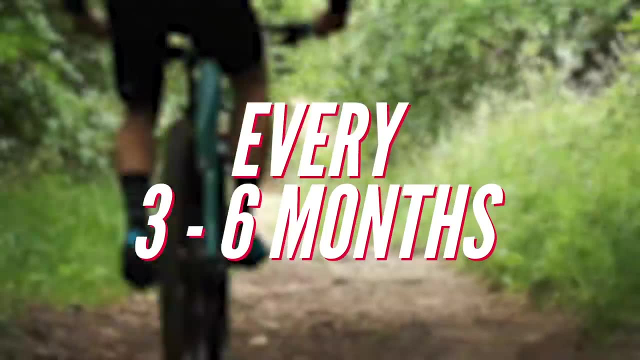 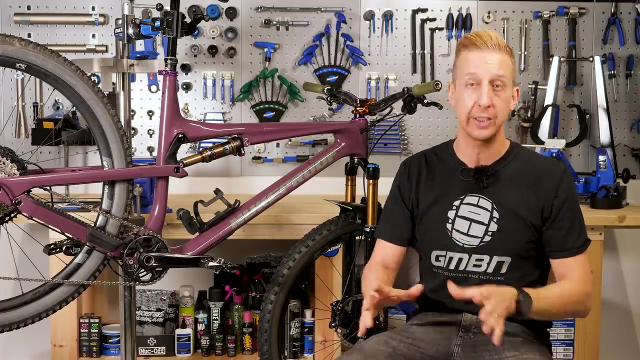 anywhere near your brake, which is obviously just on the left-hand side of your fork leg, because of course you get any oil near your front brake. it's still going to be working Every three to six months. Now this is getting pretty vague here, because this entirely depends. 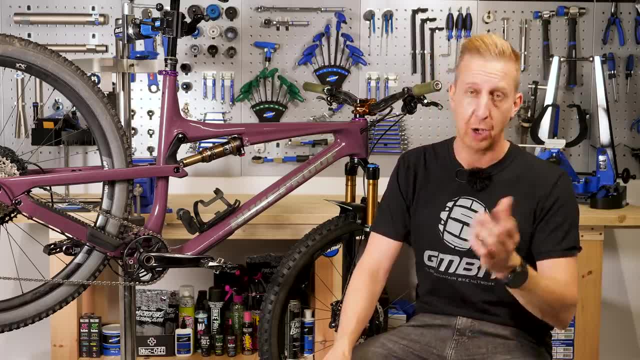 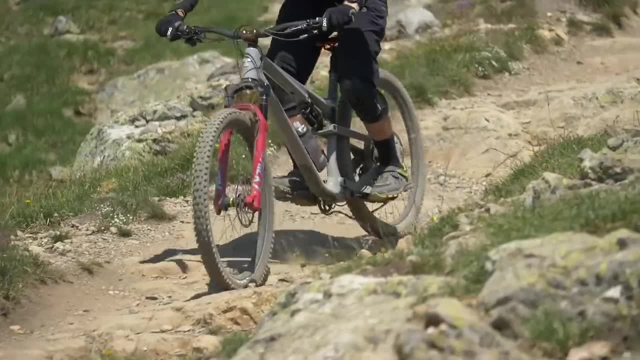 on how hard you are on your bike. If you, for example, live near Whistler or some sort of alpine bike park, you're probably going to need to do this level of servicing every month, not every three to six. Likewise, if you live somewhere that's got very sandy, gritty dirt. 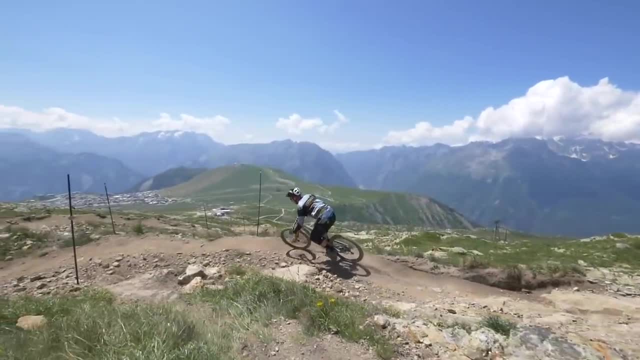 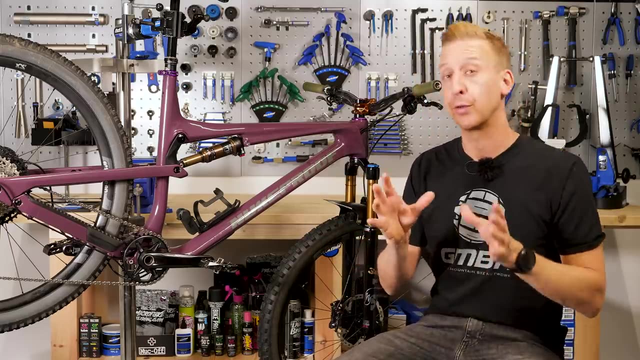 the same thing. you'll actually smash through your transmissions far more frequently. You've got to apply this to yourself. Suspension units we'll look at first. Every three to six months roughly, you're going to need to do a shock, air sleeve service and the same on the fork. 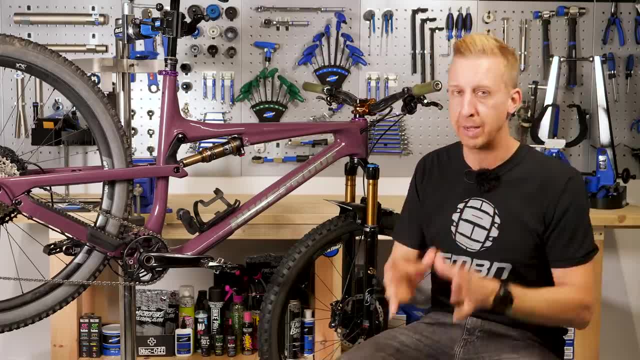 which is a fork seal. You're going to need to do a shock air sleeve service and the same on the fork, which is a fork seal. Now, the servicing intervals recommended by manufacturers does differ, so you do have to use your common sense here Now. Fox recommend every 30 hours. 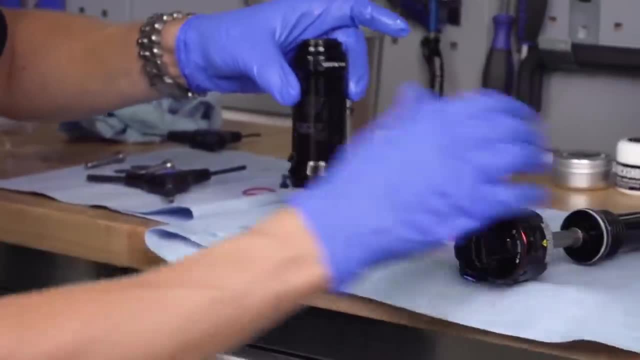 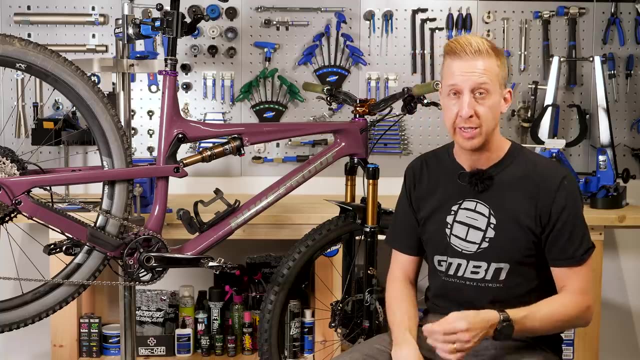 to do the fork and the shock service RockShox recommend every 50 hours. Now again, this totally depends on the way you do things, but actually I do mine far more frequently because it means that they work insanely good all of the time. They're very 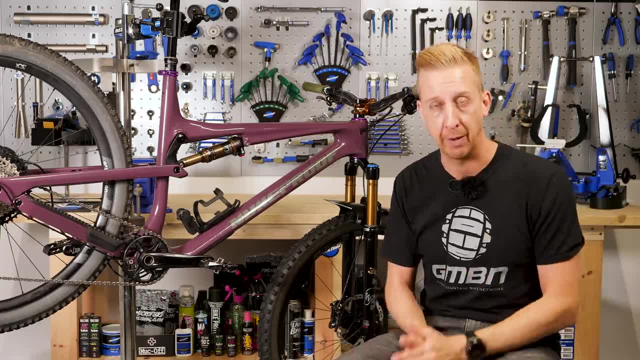 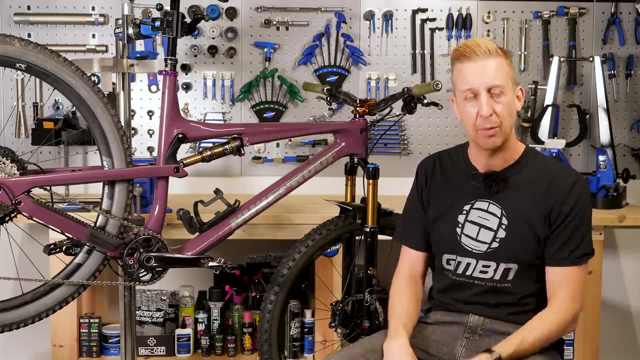 supple. Now. an easy way to tell if yours do need a bit of work is they might not fill in particular the fork. It might not feel quite responsive on the smaller bumps. It might just feel a bit sticky or a bit slower than usual. If that's the case, then they're probably quite dry and they're going. 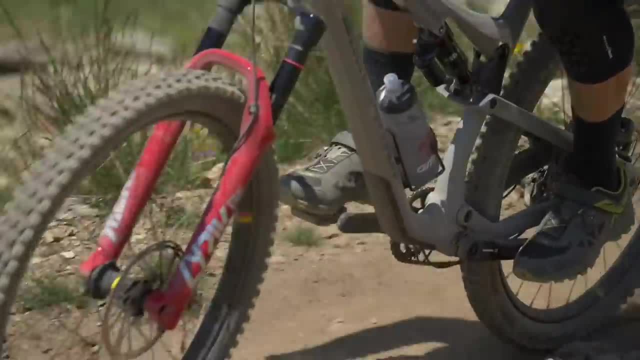 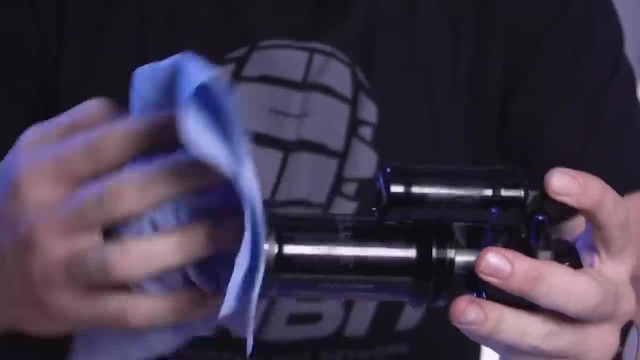 to need some love. Definitely treat them to a fork lower leg service, whether you do it yourself or you send them to your local friendly suspension tuner. The same applies to the rear shock. Very simple to do an air sleeve service yourself. We've got videos for that. 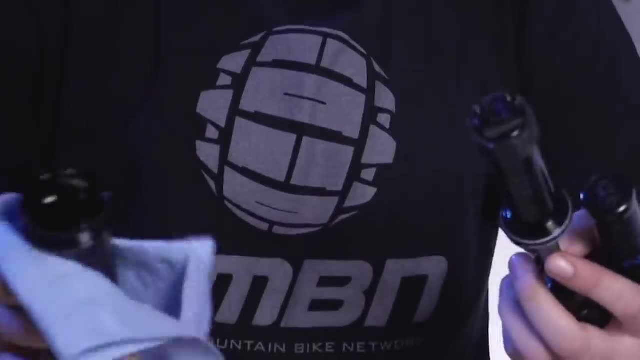 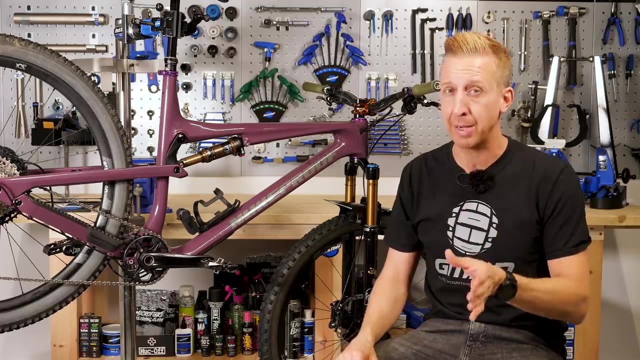 but if you're not confident in doing that, book in with your suspension tuner Checking your frame bearings for play. Now, if you're a cross-country rider, you might only need to do this annually, and maybe not even as much as that If you're really hard on. 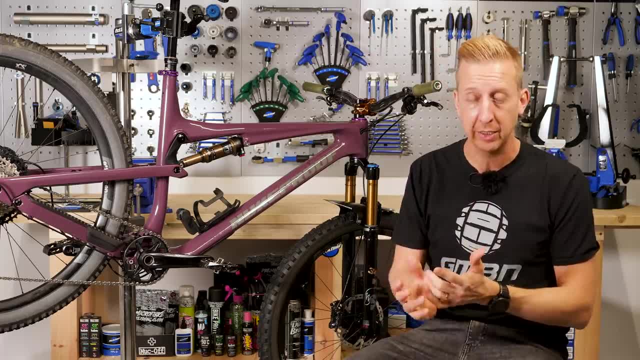 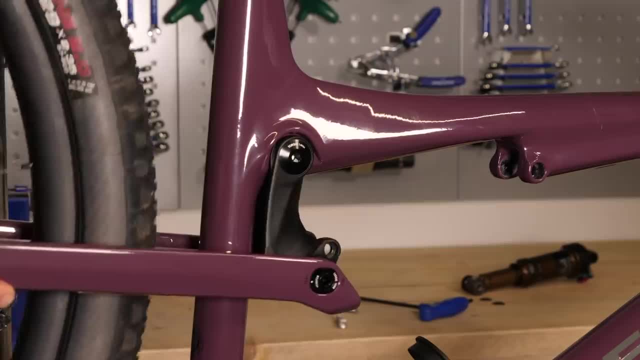 a bike. if you ride a lot of downhill, you do uplift. if you're doing jumping, anything like that, that's really excessively hard on the bike. you're going to go through frame bearings. A good way to check them is by taking the shock out and cycling the rear end through. Sometimes you can. 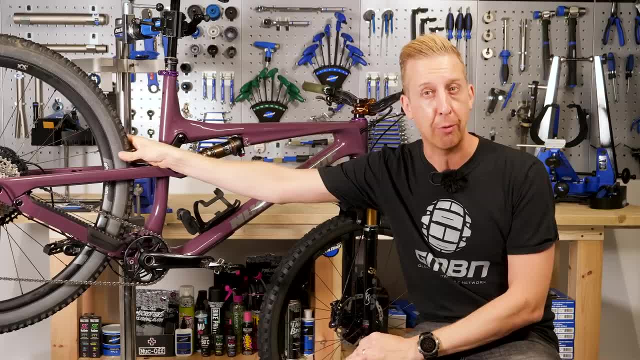 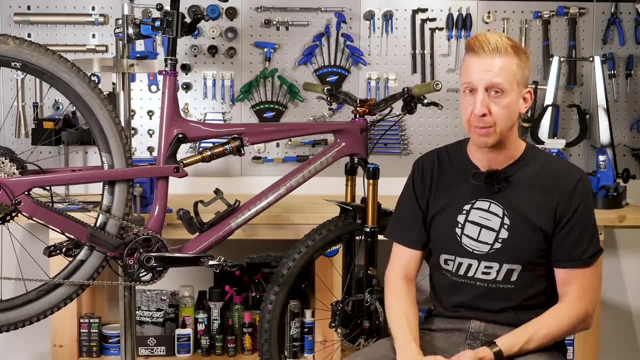 feel if they're notchy. Sometimes you better feel if there's any play. but don't be confused with play in the rear hub or the wheel. You should be trying to move the frame itself. It becomes pretty easy. You can normally, if you just pay a bit of close attention, work out where it's coming from. 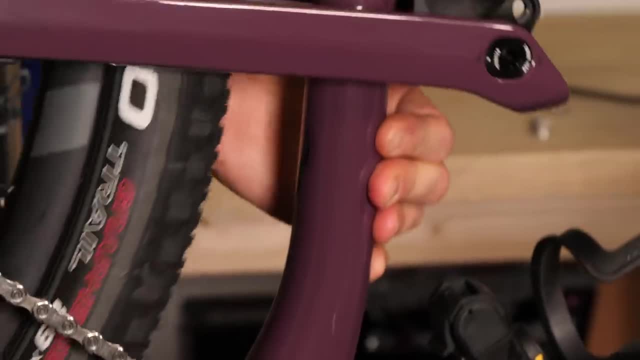 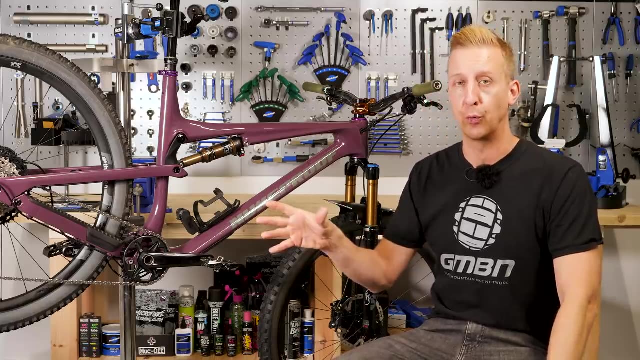 It would normally be one of the main pivots as opposed to one of the smaller pivots, but just take your time working your way through those. Now. I'd say roughly every six months or so you want to be stripping down your rear hub. 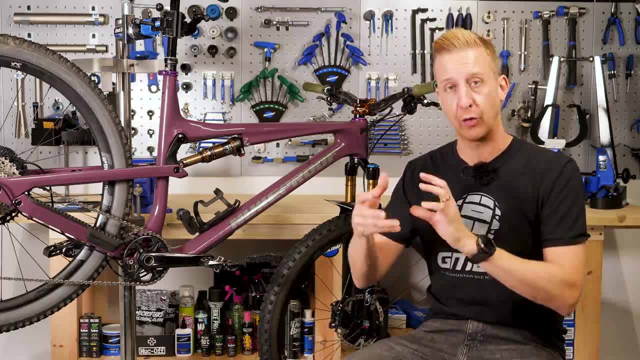 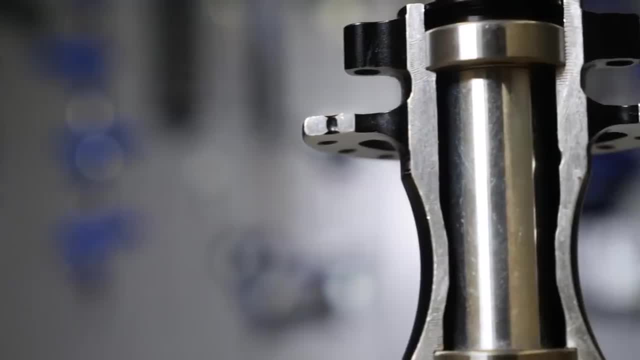 Now in your rear hub you have the free hub mechanism. This will either be a ratchet system or a system of pulls. Either way, gunk gets inside and it slows everything down. In the case of pulls it can actually be really bad, because if they stick they won't engage properly. 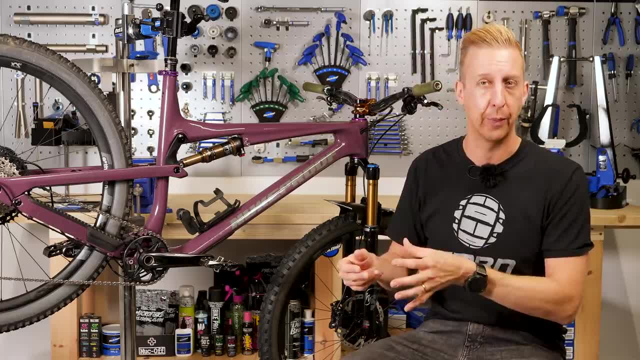 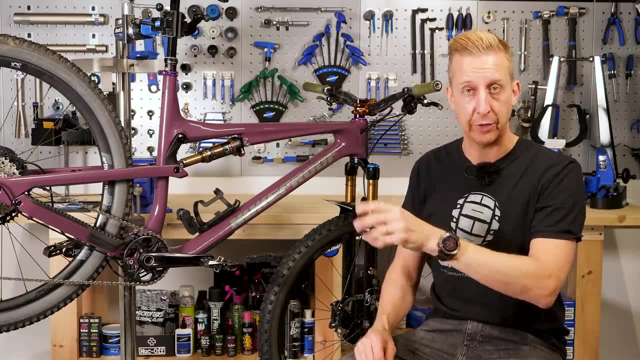 whereas with the ratchets it just eats them up a little bit. They'll continue to work no matter what, but things get slow, you get more drag, you get more friction. It's really not a hard job to remove the cassette. You'll need a chain whip and a cassette tool. Remove the cassette. 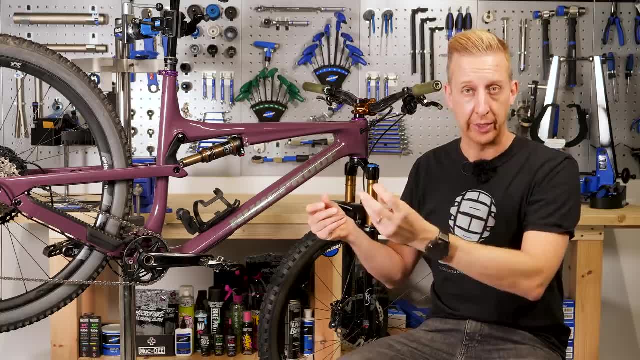 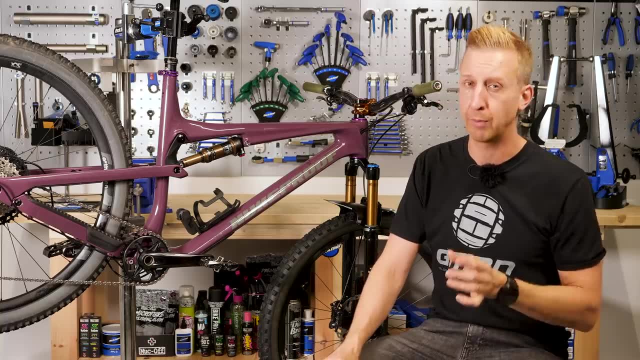 from your bike then basically take the hub apart, slide out the cassette body and give it all a good clean. Now one bit of advice. unless you're using a particular grease that's recommended for your hub, like DT, have a special grease- I think it's actually called special grease- for their. 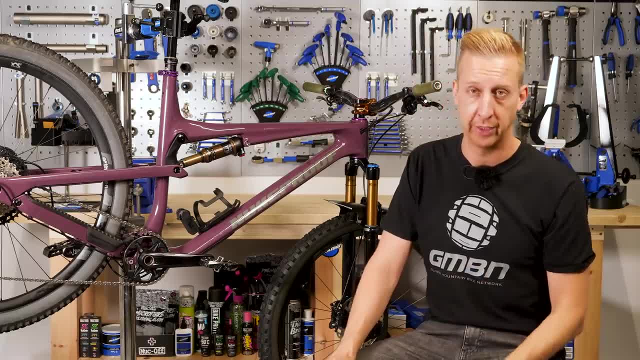 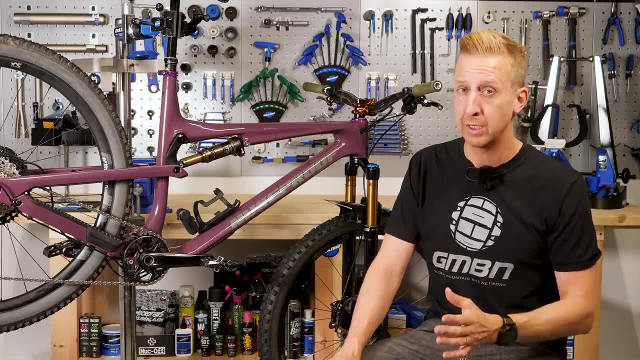 ratchet mechanism. I'd actually recommend using an oil rather than a grease on here. If you have to use a grease, a suspension grease that is very runny and very, very thin would be better. You don't want to have something thick that's going to slow it down, or even have any. 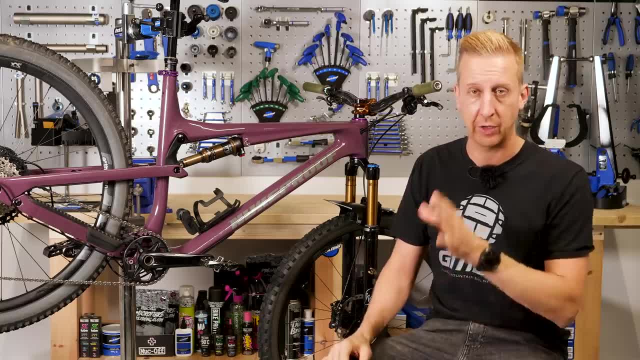 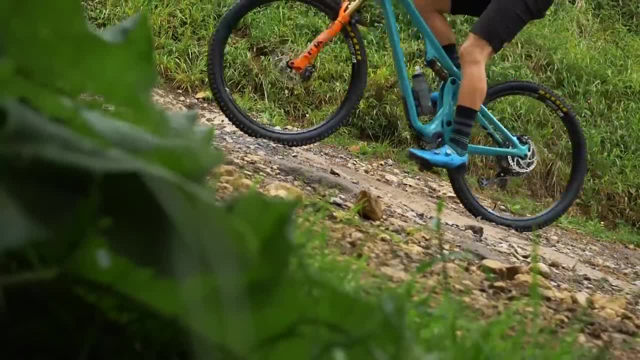 risk of congealing and making the pulls stick. Something nice and thin. give your hub a bit of love. Think how much abuse your rear hub has. The front has barely got anything to deal with. by all accounts, The rear. you're putting all that torque, all that power through it. 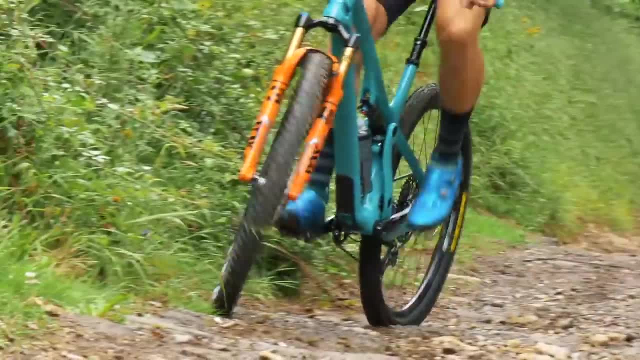 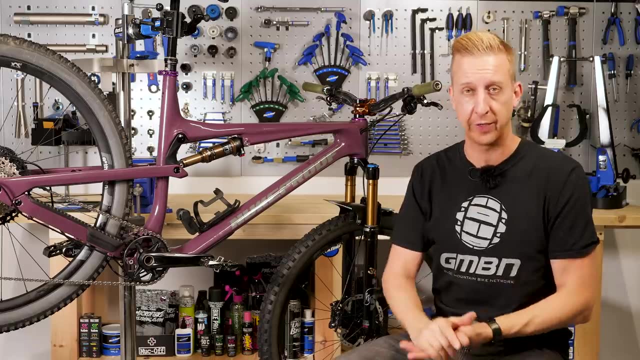 all your body weight constantly. It's no wonder it needs a bit of love Every six months for that one. Next up your headset bearings that sit either in the frame, like these ones, or they sit in a cup that's pushed into the frame. 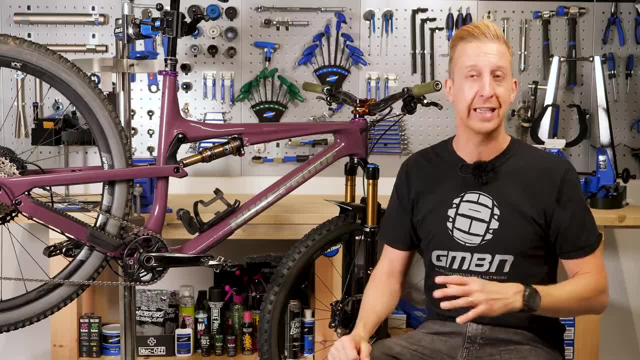 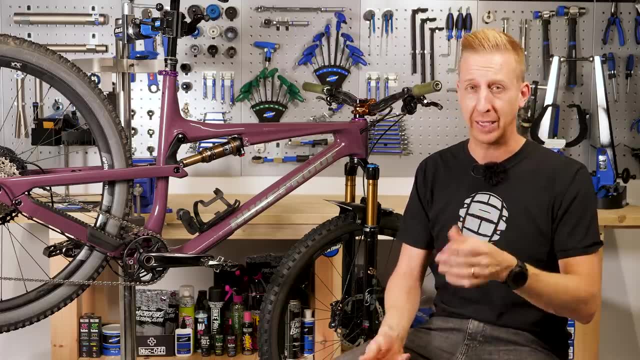 Either way, it's one of the parts of the bike that I think we're all guilty of basically leaving until it becomes a problem. Your steering can get notchy and the bearings can disintegrate from repeated impact. I've seen Blake destroy lower races of bearings- Nothing to do with the 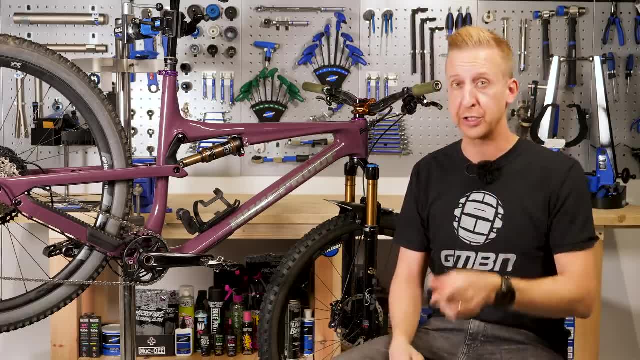 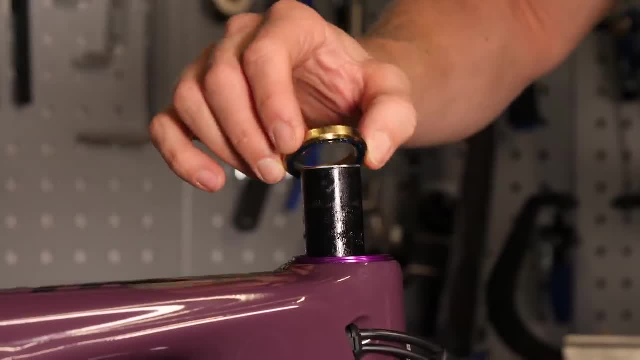 quality of the bearings just from the way he rides the bike so hard. If you're into jumping, chances are you've done this as well. Definitely take off, see the whole front end of your bike there and inspect the bearings- I'd say every three to six. months- probably six months- is good. If you're in the UK in winter, you probably want to be doing this every couple of months. Again, it does depend on the conditions, because water and moisture gets in there. It gets rid of all the grease that's in there, naturally, and you're left with bearings that 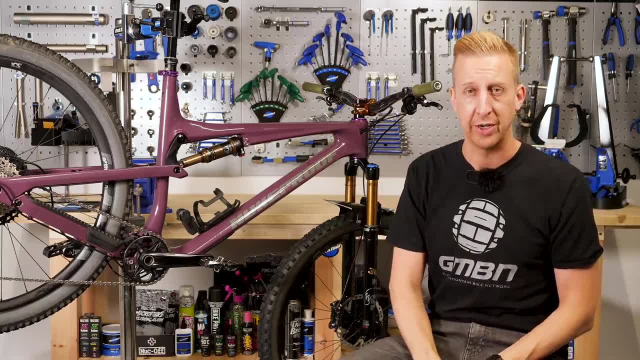 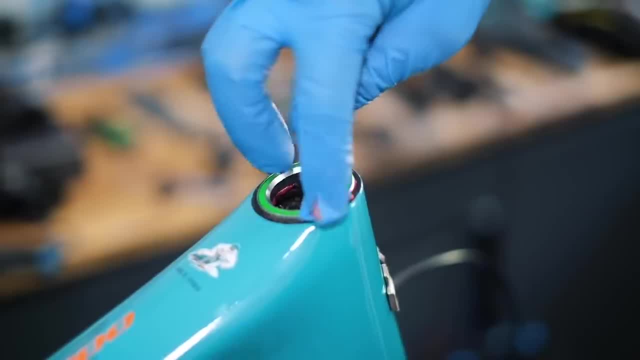 are just basically rattling around. They'll just grind themselves to nothing. You can replace bearings really easily. Some bearings, you can look after them and put some fresh grease on. You'll have to decide which variety you have when you take them apart. 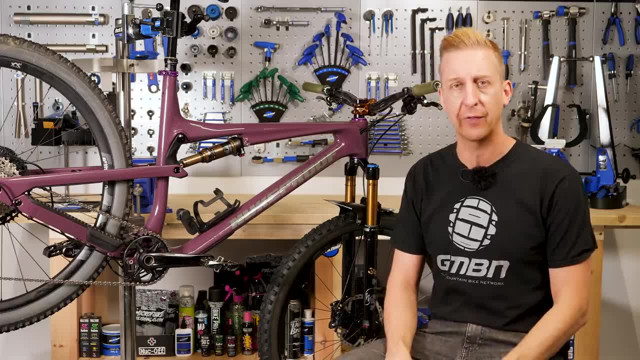 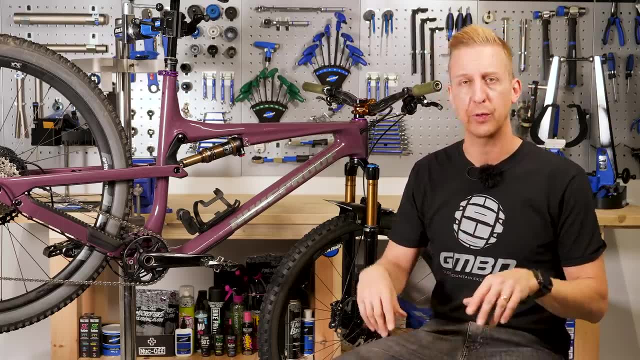 Bleeding your brakes. Now, unless you're particularly unlucky or you have an unlucky brake, it's pretty much something you're doing on an annual basis, which we'll get to From time to time. it's possible to have maybe a brake lever that needs a bit of pumping before it feels good. 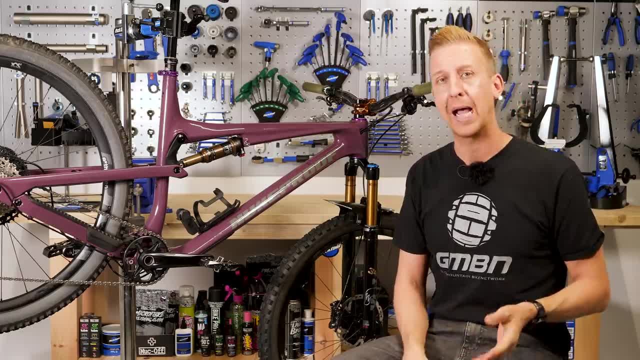 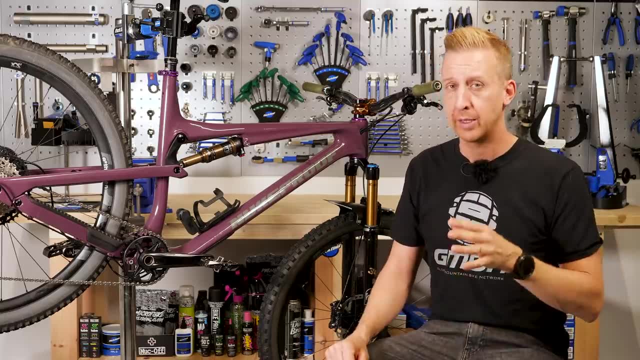 It might come to the bar a few times. I'm sure some of you know that feeling. Perhaps if you store your bike upright you'll notice when you get it down the brake goes all the way to the bar. Same thing got to pump it a bit. It might not necessarily mean you need to do a full bleed. 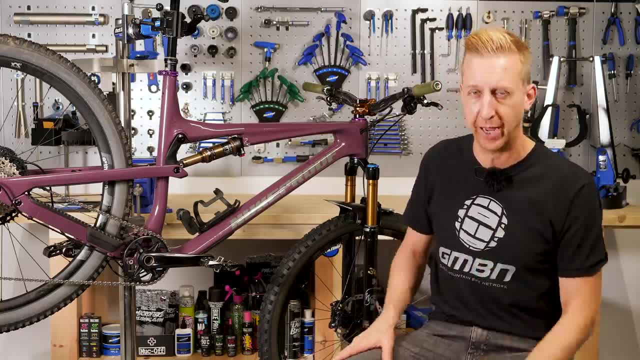 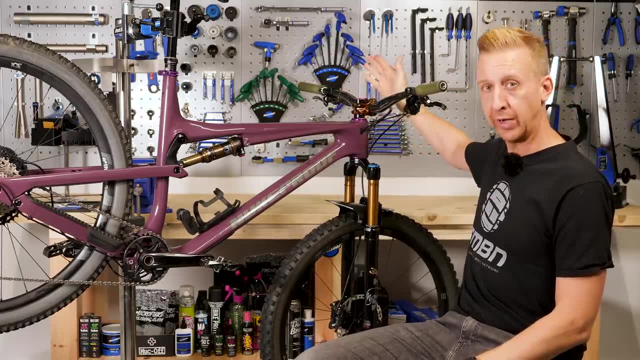 You can do a mini bleed. This is a bit of a cheat for reversion. It's a good little hack If you can. let's just say it's your rear brake- Put your brake lever down into a vertical position and then put your bike up on the back wheel. 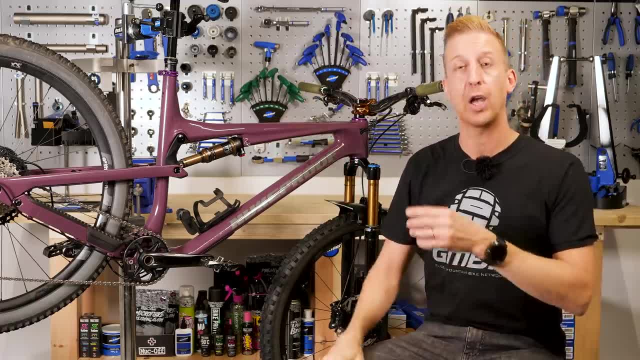 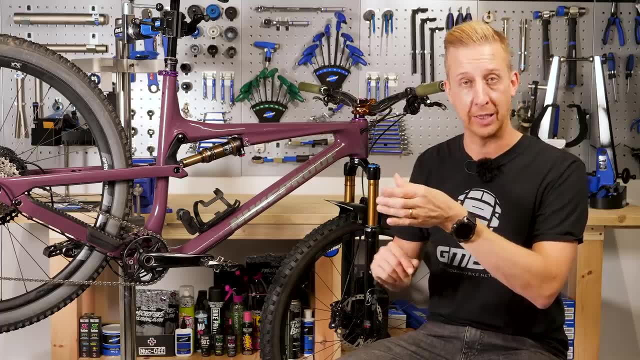 If you're hanging your bikes up like I do, it works really good. doing it like this, you're going to basically open the top of the system. If you leave it overnight, you'll find that those air bubbles will migrate to the top and they'll pop out the top and disappear. 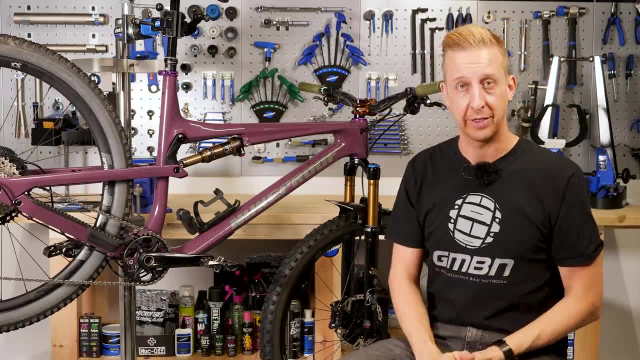 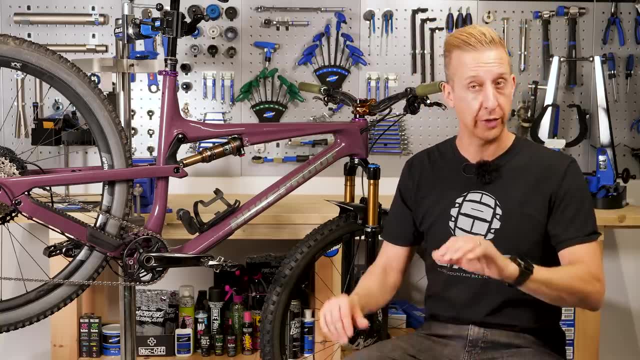 All you want to do then is just top up on the fluid and replace the bolt into the top there. If you're hanging your bike upright, you can do a full bleed. It's a bit of a cheat for reversion. You're replacing that air with a bit of oil and you'll find it feels pretty good again. 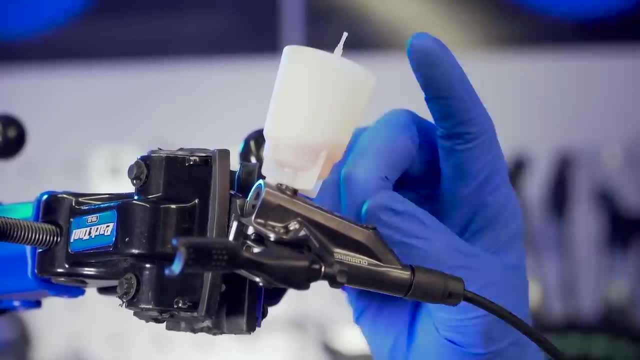 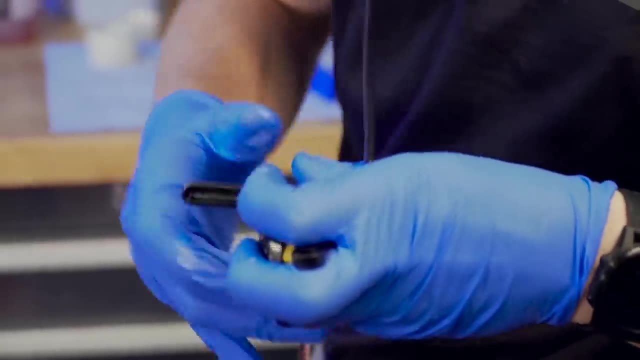 but it's not a way around. a genuine brake bleed. If your brakes need bleeding, just do it. It's always easier than you think, always takes less time than you think. yet it's one of those things that most people put off until they really need to do it. 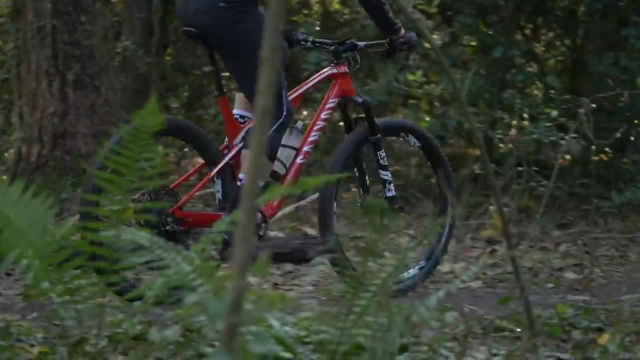 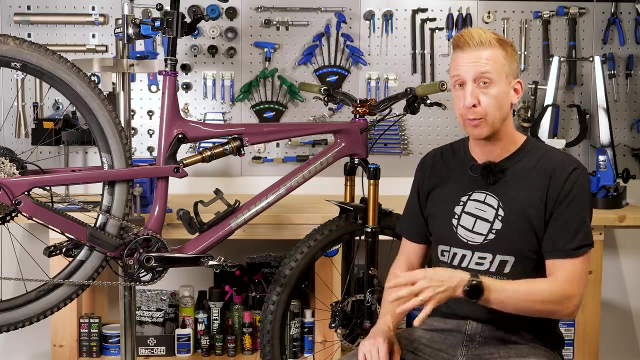 Annual Service- Okay, annually. Now this is the big service. If you're going to send your bike to a bike shop and it's a full suspension bike like this, they're probably going to want to do in an annual service shock, a fork and a seat post in addition to everything else. 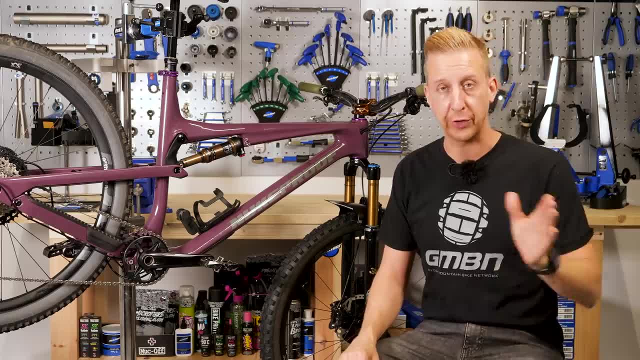 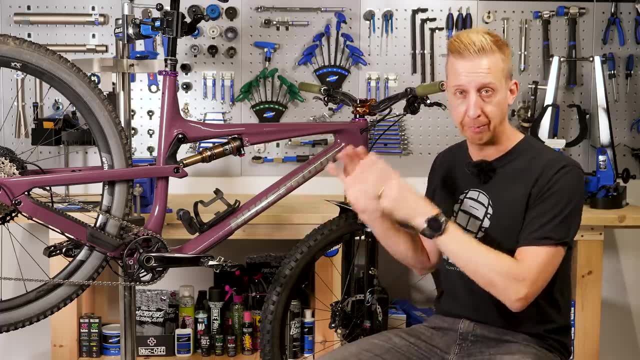 This is why I think it's really important to highlight the fact that there's jobs that you can do throughout the year on a daily, weekly, monthly and three to six monthly basis, aside from the big annual service Now every 100 hours or so. 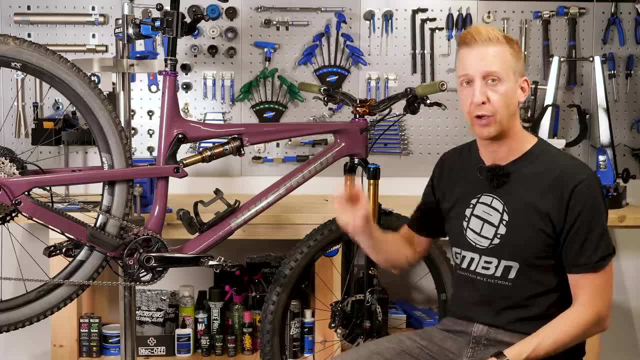 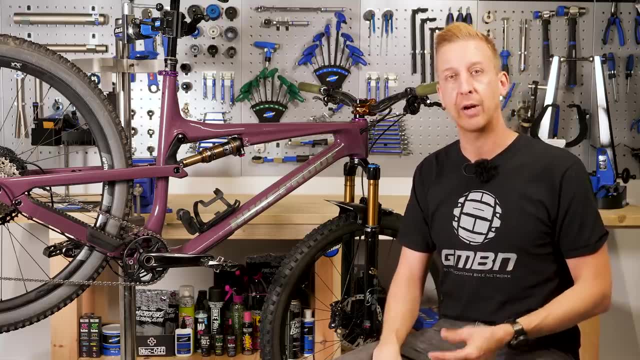 your forks, your shock and your seat post will need a proper service, Starting at the seat post. if it's a hydraulic post like the RockShox Reverb, every 100 hours or so of riding they recommend a full system bleed. At the same time, you want to be checking for excess play. 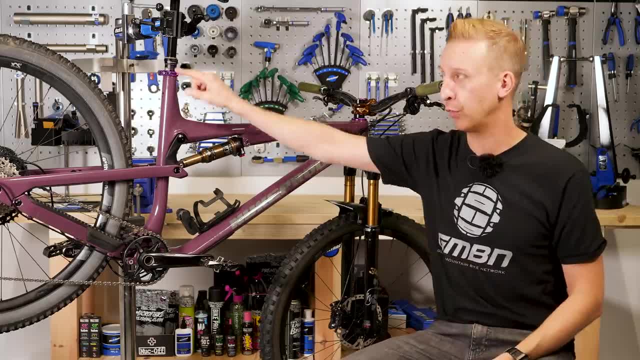 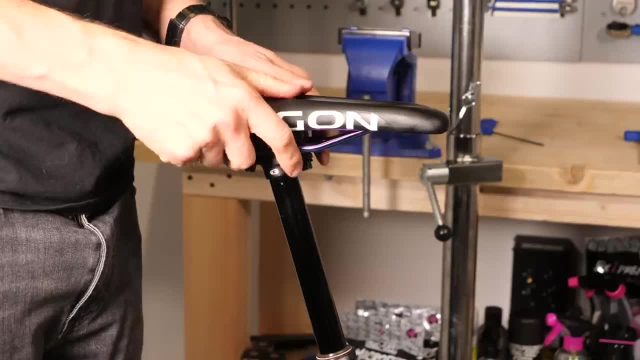 Now, all dropper seat posts have a system of keys. They basically have some grooves on the inside and they have brass keys that run down those grooves. That's what stops your saddle just moving sideways. if you think it's just a round post, basically They are designed to wear out. 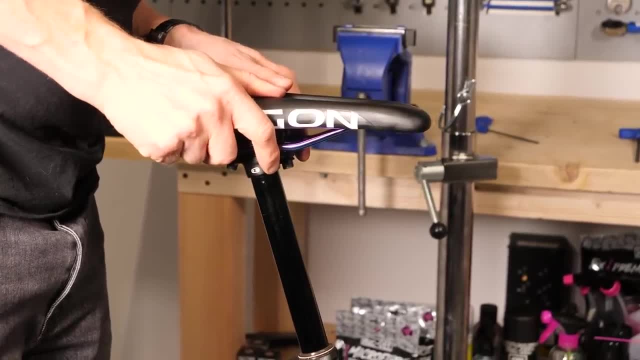 They're a consumer-friendly system. They're designed to wear out. They're a consumer-friendly part. Don't worry about that. If it gets a bit baggy, you just need to replace those brass keys that are on the inside. A full seat post rebuild is recommended if you have a hydraulic one. 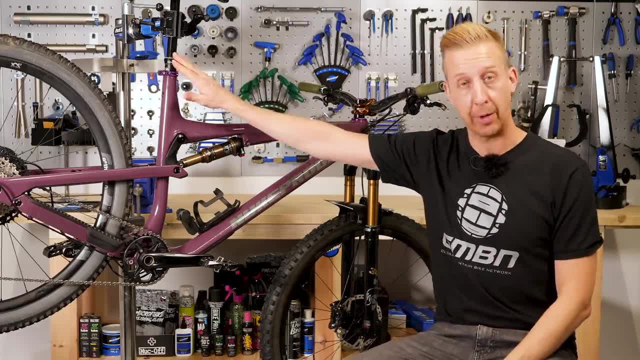 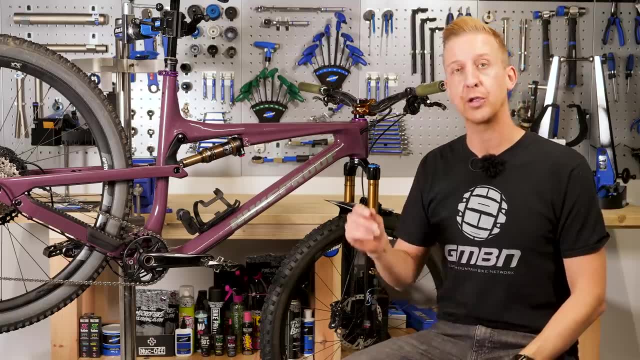 annually. If you have a cable-operated post like this one, they come in a few different varieties- You can do a basic service where you take it apart, clean it, grease it and put it back together If the actual unit itself fails on the inside. these ones have a sealed cartridge on the inside. 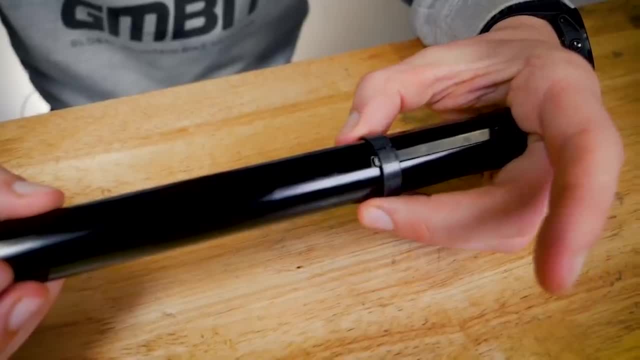 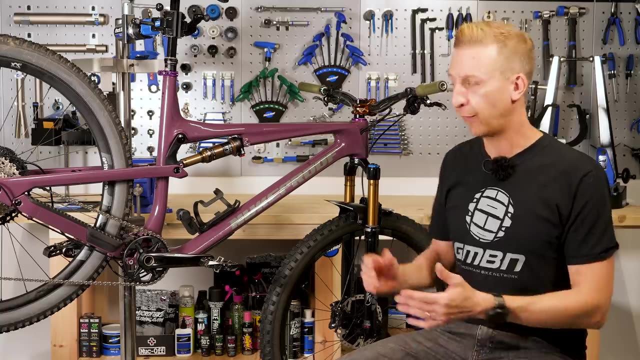 which you just replace the cartridge. You don't actually service anything. There's various different options out there. Just look into the particular one that you have. Some are user serviceable, some are not. Forks and shocks. Now, every 100 hours or so, you need a proper damper. 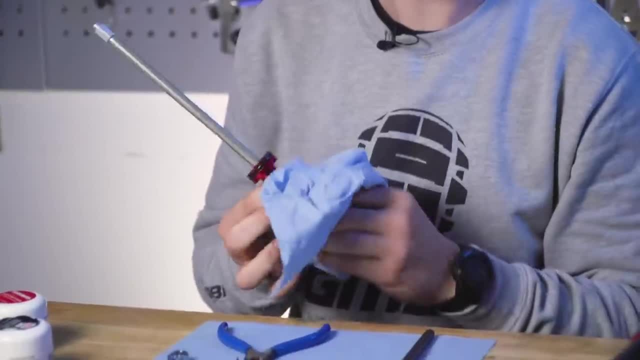 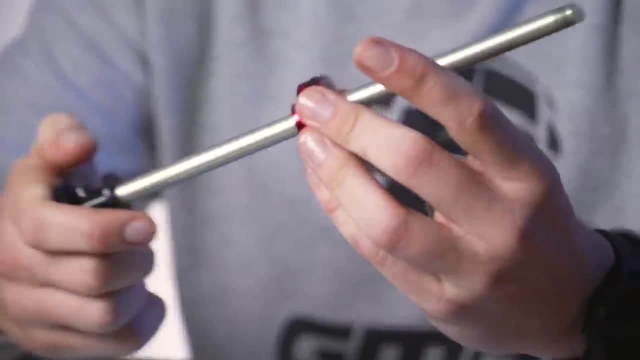 service. That's an internal service. It's not just a case of taking the air sleeve off, giving it a clean and putting it back on. Nor is it a case of just taking the fork lowers off, cleaning them and putting some fresh lower lubing. This is taking apart the damping unit on. 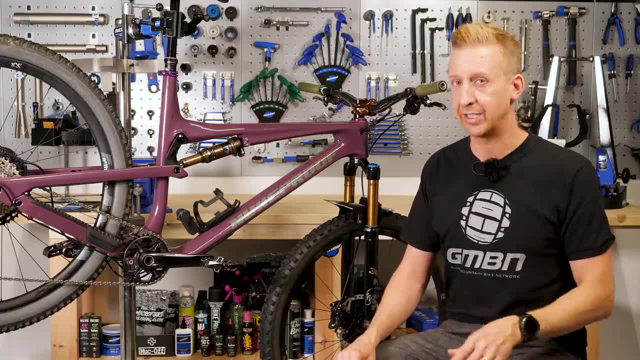 the inside. Now, I'm sure for about 90% of people out there, this is not the sort of thing that you do. This is what your suspension tuner's going to do. This is what your suspension tuner's going to do. This is what your suspension tuners are for. Even most bike shops will send these units away. 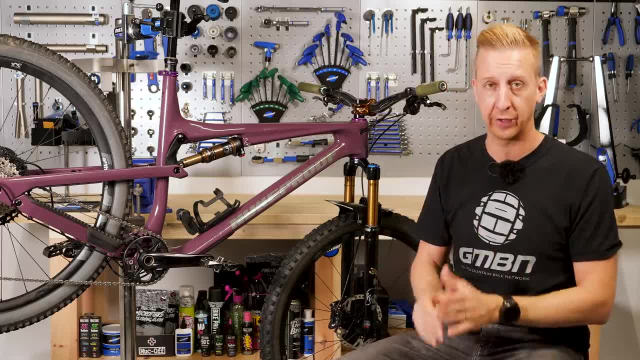 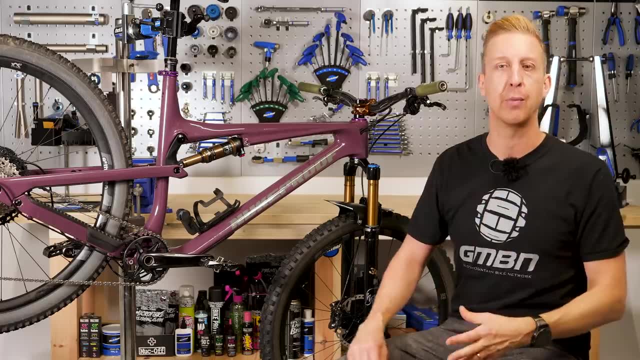 to suspension tuners. After all, that is what they do day in, day out. This is also a great opportunity for you at this point to have yours custom set up for you. If you perhaps found there's certain elements of your bike that you don't like, you can have it. 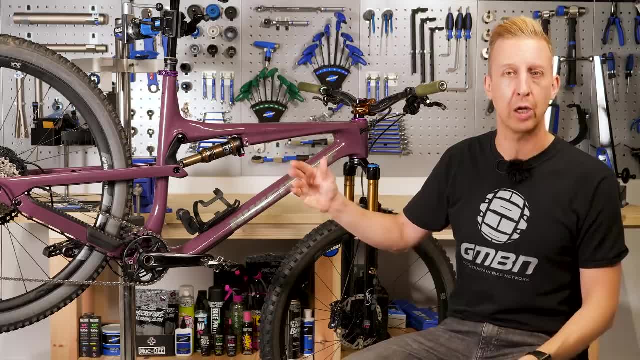 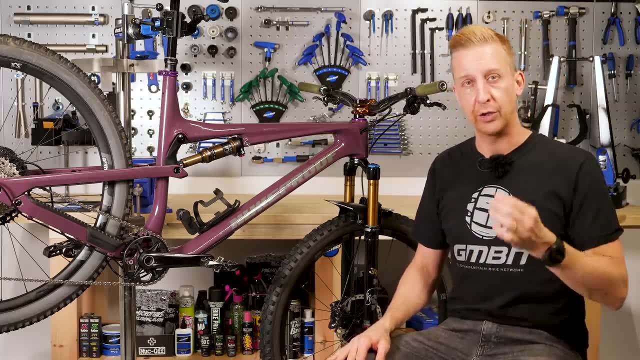 tailored around that. Maybe your back end bobs too much when you're climbing. when you've got it on the open switch, You can have some more compression put into the shock at this point. It's always good to get a good relationship with your local suspension tuner and they'll be able to talk you. 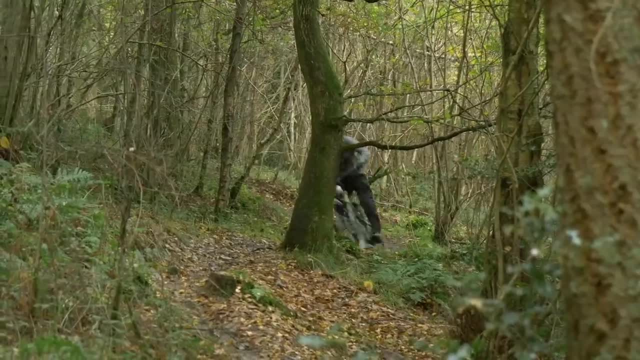 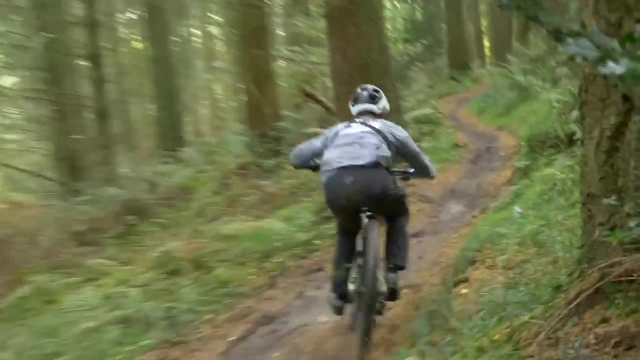 in style with your bike and sort it out for you. Now also, bear in mind you can also ride a fork or a shock for several years without having to do any of this stuff and you might get away just fine. Can I just tell you that there's a lot of damage that occurs on the inside of forks and 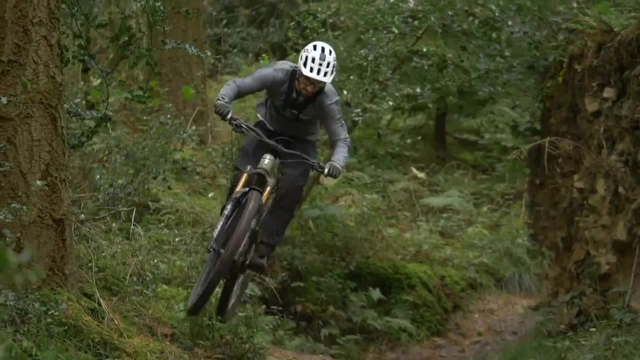 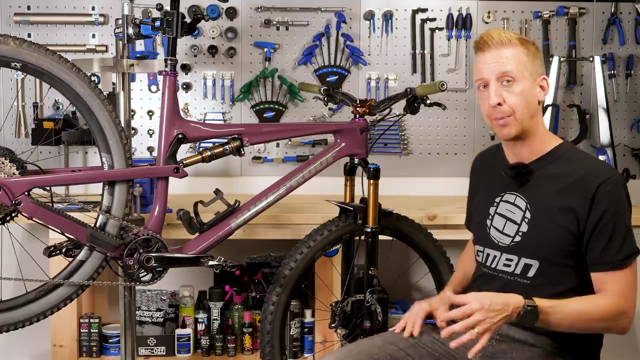 shocks that you might not know about. Those things can lead to much more expensive items at a later date. For example, a classic one is the inside of these tubes being scratched. If that happens, they're not going to basically keep the air on the inside, but to replace that part. it's not just 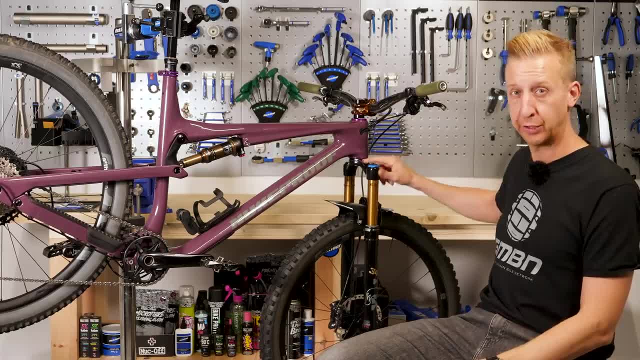 these tubes. They're going to be scratched. They're going to be scratched. They're going to be scratched. They're bonded into the crown, which is part of the steerer tube as well. That's the whole upper part of the fork. The whole upper part of the fork can cost nearly half as much as buying a new fork. 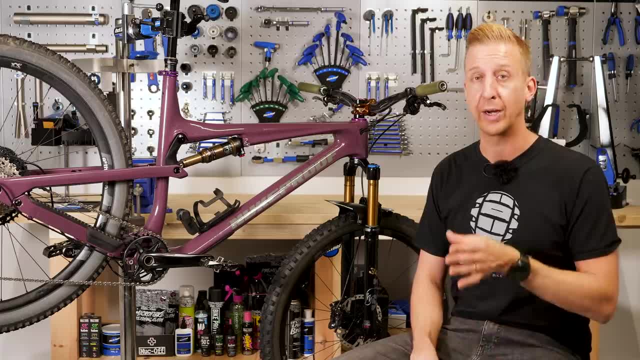 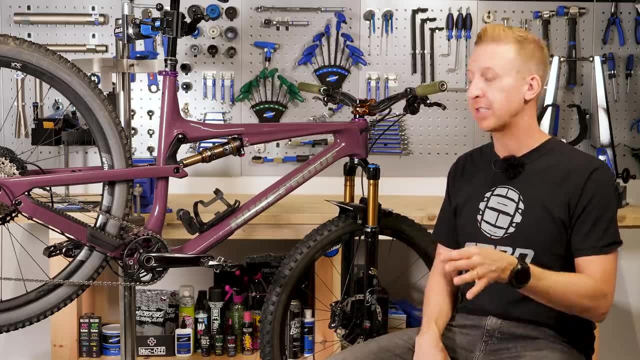 You don't want that to happen. That is definitely something that can be prevented by regular servicing. I just think servicing will make these things last longer. It's all about longevity, so just take care with that. Don't be surprised when they do a full service. 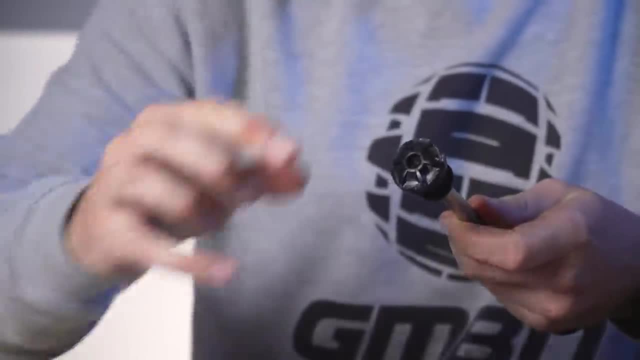 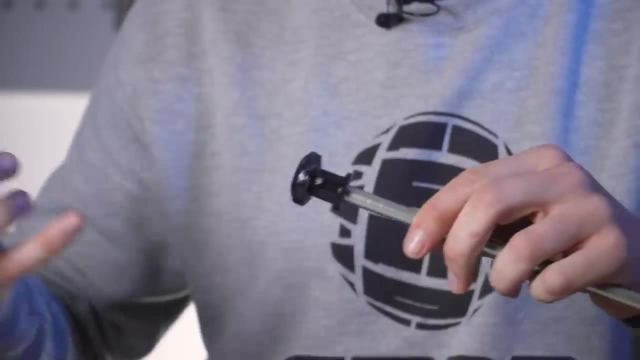 if they're things like the seals, the bushings on the inside and a few other components like O-rings and stuff that will need replacing. That's pretty common, along with an oil change Brakes. Now, you should always bleed your brakes once a year, I think. Now. with DOT fluid. you actually should definitely bleed them once a year because DOT and mineral fluid are very different. DOT fluid actually ingest moisture over time and air can get into the brakes. As a point, you should flush your whole system through. get some fresh oil in there. 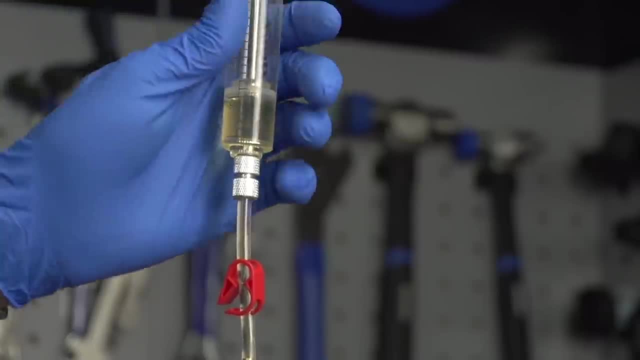 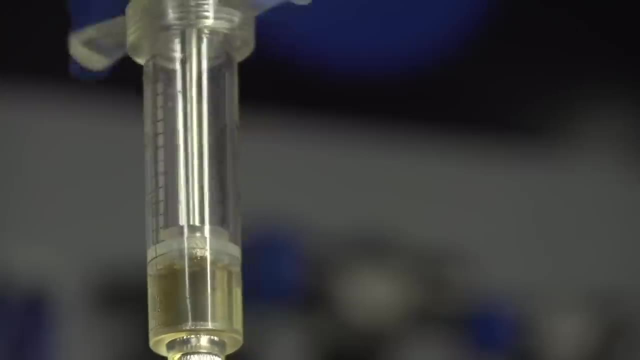 Something very important to note with DOT fluid is you should use a fresh container each time. The second you open a container of that, once you put the lid back on it, it can still technically ingest moisture into it- A fresh bleed- once a year If you've got two or three bikes with them. 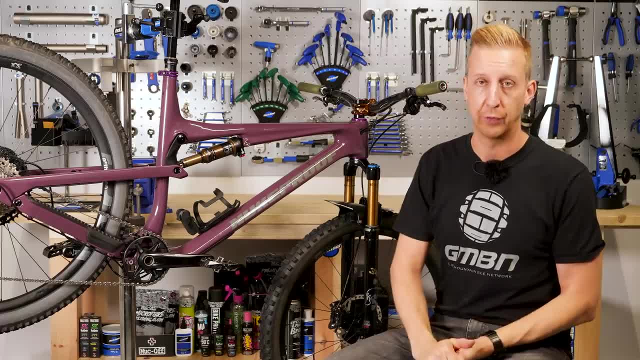 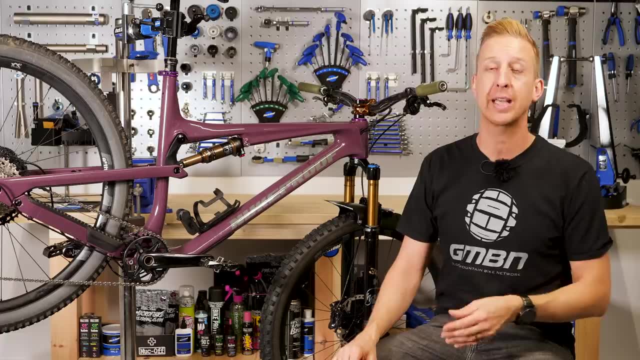 do them all at the same time. Use up that pot of DOT fluid you've got. With mineral brakes like Shimano or Magura, for example, it's less of an issue. However, the fluid can still get a bit manky after a while, so I definitely recommend an annual system bleed.